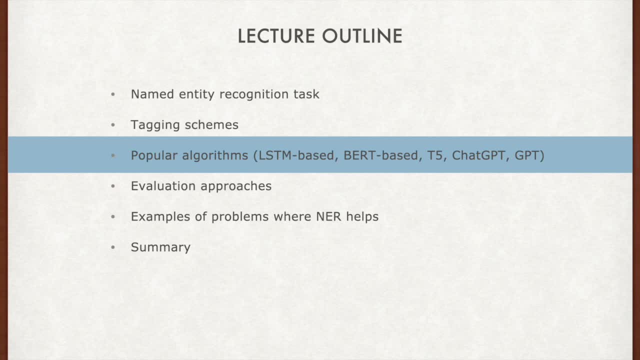 The third section of our story refers to a subset of popular algorithms that are used to create labels. The third section of our story is regardable to a general environment. The third section of our story is Appreciative demeanor et al Each 누. 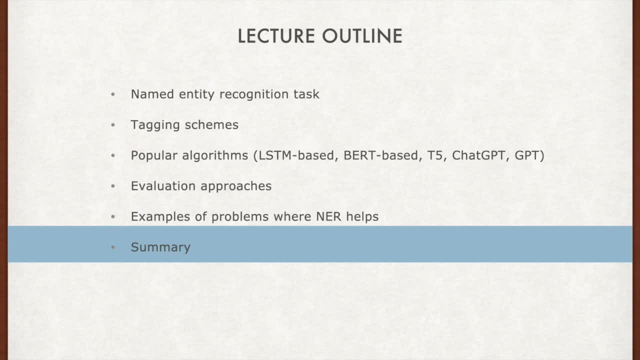 And finally, we will summarize our lecture. In previous lectures, we discussed the idea of generating context-aware word representations use tasks. Frequently, we discussed the idea of generating word embeddings that could be aggregated into one vector for the purpose of the classification task, which focused 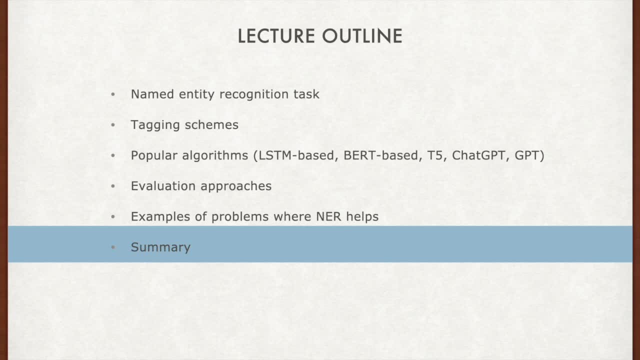 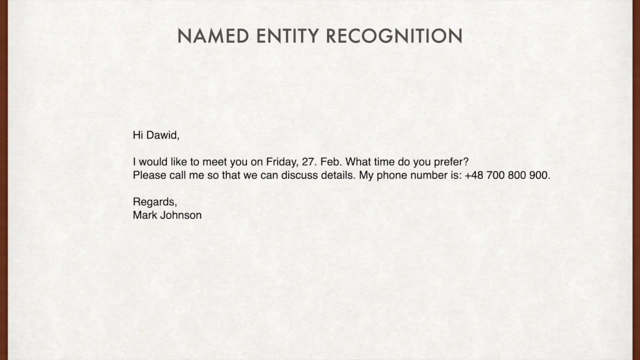 on assigning one or more labels to whole documents. Named entity recognition is a similar task of assigning labels to texts. However, instead of labeling whole documents here, we would like to extract short fragments of text and assign labels to them. Consider the following example: You receive an email. 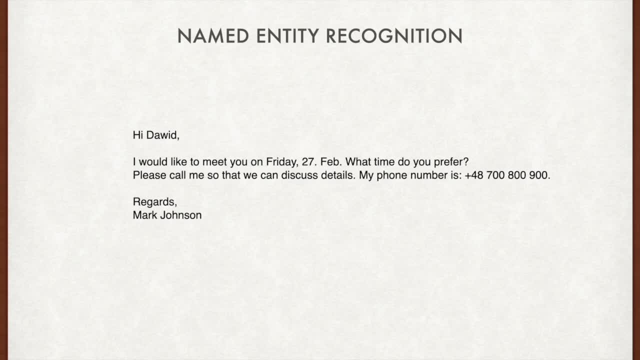 Hi David. I would like to meet you on Friday 27th February. What time do you prefer? Please call me so that we can discuss details. My phone number is: and here is the phone number. Regards: Mark Johnson. In this email we have. 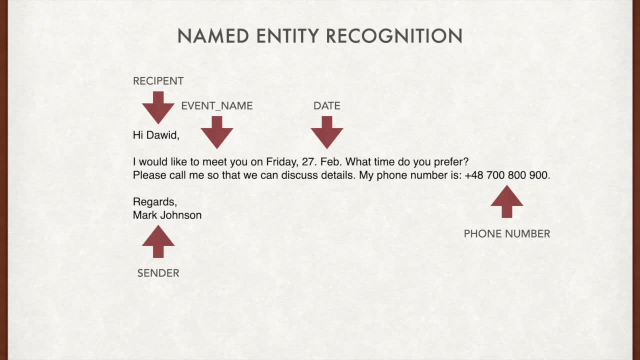 several interesting pieces of text which could be interesting from our perspective. For example, we have a date- Friday, 27th February- a phone number and the full name of the sender here: Mark Johnson. We could even identify the recipient here: David and. 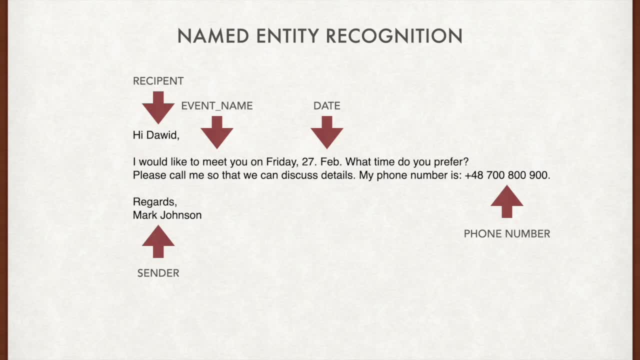 even extract the word meet as the event name, because this is some kind of an event. All those interesting fragments of text might be interpreted by our products. If we can detect phone numbers on phones, we could provide a functionality in which you tap on the number to make a call If a given phone number is 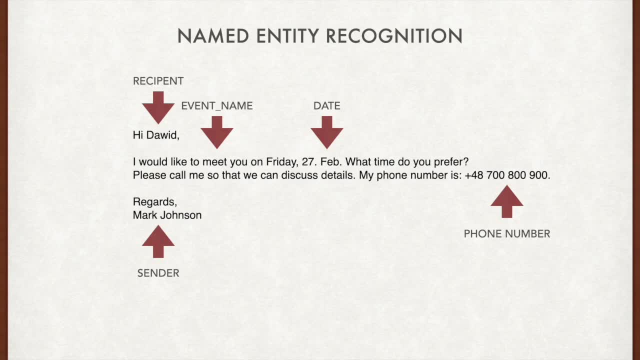 not present in your contact list. we not only will have the phone number but also the full name of the sender here, Mark Johnson. so that we can get this option here raised, We could suggest adding Mark Johnson to our contacts. Also, Being able to detect dates shared on the phone, We can also add the contact number to the. 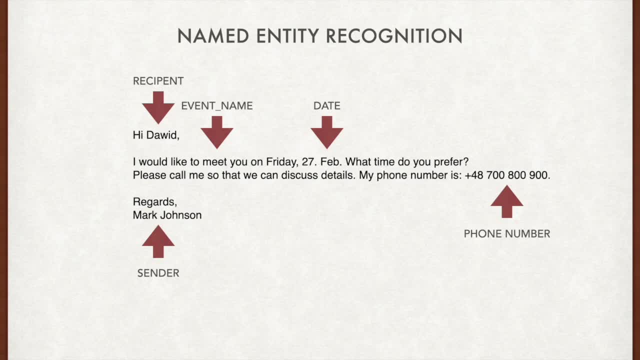 contacts- if it would be Mar saint mark- and make contact certificate. You can also use phone number. It's quite easy to be able of adding to particular contacts. We could add some events to our calendar with only one click. The story of this email shows us the context of today's lecture. 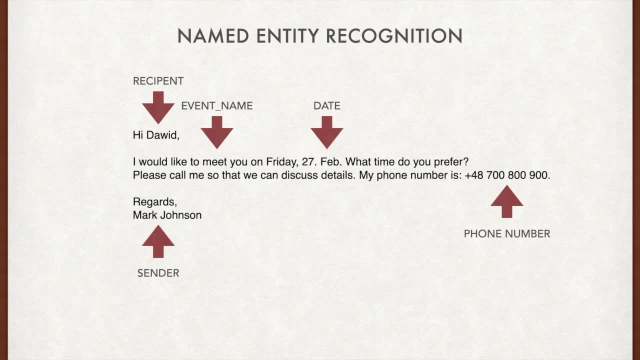 Named entity. recognition is the task of identifying interesting fragments in texts and categorizing them. The list of categories we would like to extract is defined by us and most frequently we used methods of supervised learning to teach the model how to identify the fragments, based on a set of examples provided in the training set. 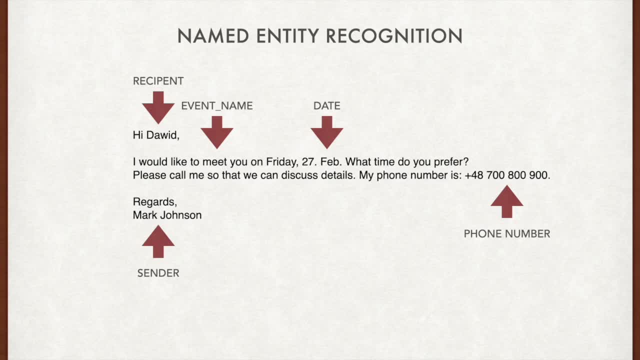 Here in this slide we observe five distinguished named entity types – recipient, event name, date, phone number and sender. All of them represent categories of things that might be represented using various pieces of text. There are a lot of possible expressions referring to dates or phone numbers, and we have about. 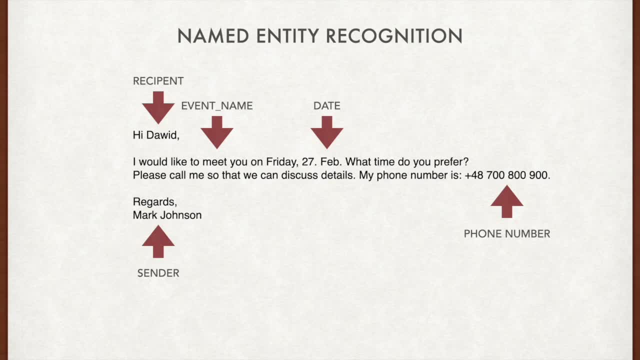 8 billion potential senders and recipients. Because those named entity types are categories of things. the way those entities are built or the categories of things they represent are different. Contexts in which they occur might help us to identify them. For example, email addresses are built in a specific way with the add character and. 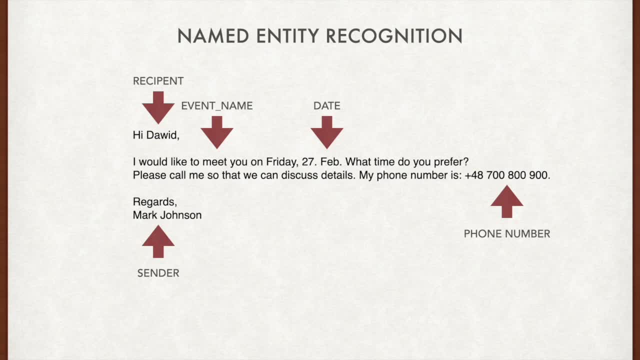 some domain name. Similarly, the phone number is quite characteristic because it consists of several digits. Moreover, the names of companies might be inferred from the context, For example the company name. When we see the reference to a company that we never heard of, we can simply look at the. 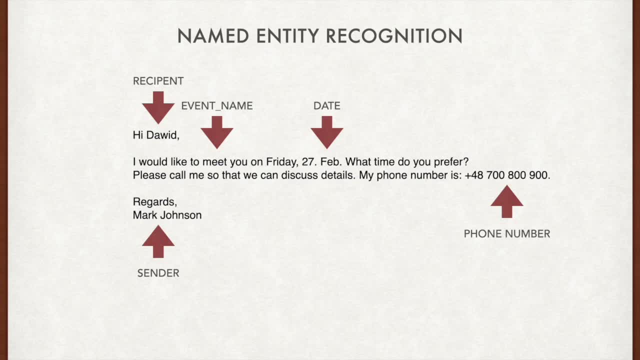 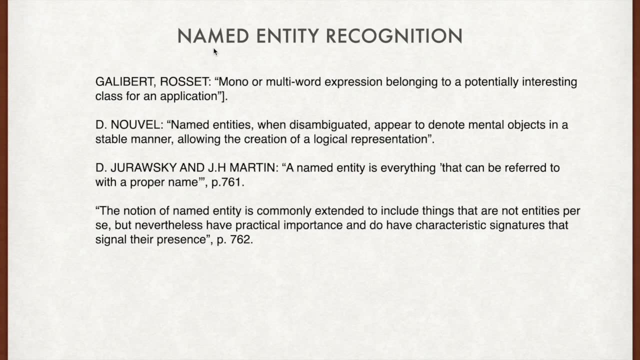 context to identify that this is probably the name of a company. There are various formal definitions of named entity recognition tasks. I gathered a small sample of those in this slide. I selected those that I found the most interesting. Galibert and Rosset defined named entities as mono or multi-word expressions belonging 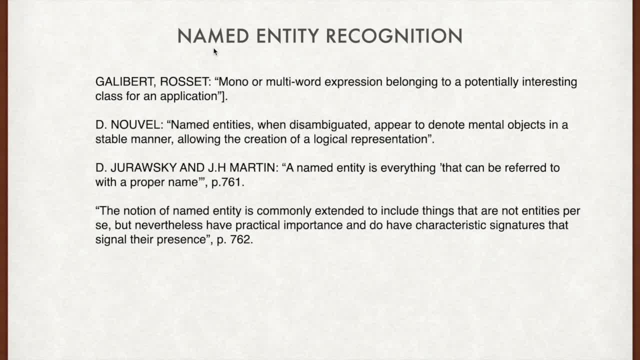 to a potentially interesting class for an application. This definition is quite straightforward, but it points to an interesting challenge we will come back to in a minute. Named entities might be composed of single tokens, but also sequences of tokens. Novel defined named entities as follows: 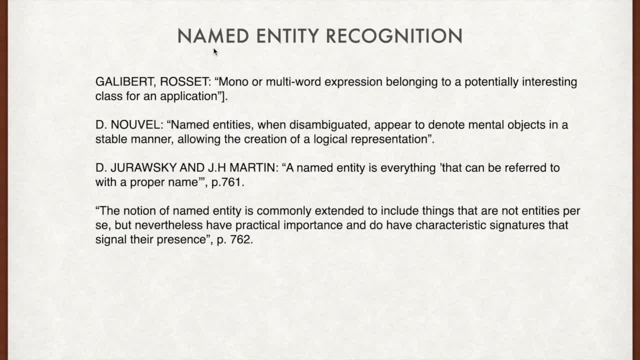 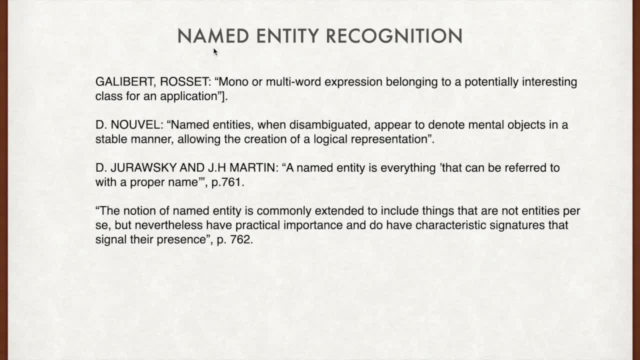 How do we approach this? They act in a stable manner allowing the creation of a logical representation. This definition emphasizes the fact that named entities refer to well-defined categories. Finally, Jurawski and Martin use the following definition: A named entity is everything that can be referred to with a proper name. and also they added: 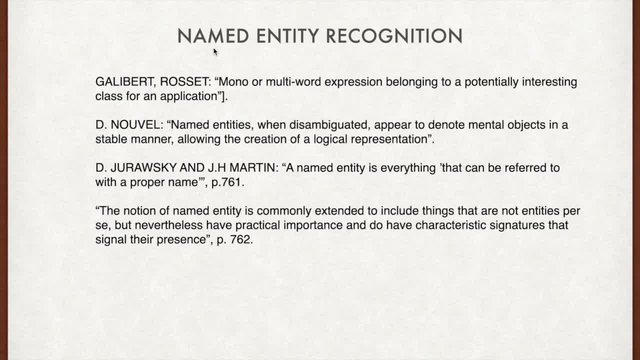 the following of named entity is commonly extended to include things that are not entities per se but nevertheless have practical importance and do have characteristic signatures that signal their presence. As we can see, those definitions focus on detecting some mono- or multi-word expressions that refer to some categories which can be named and which are useful for our needs. 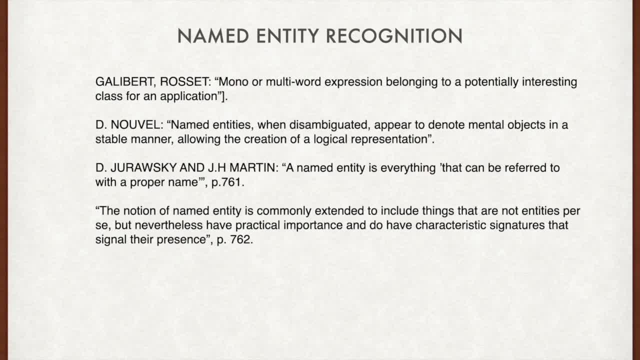 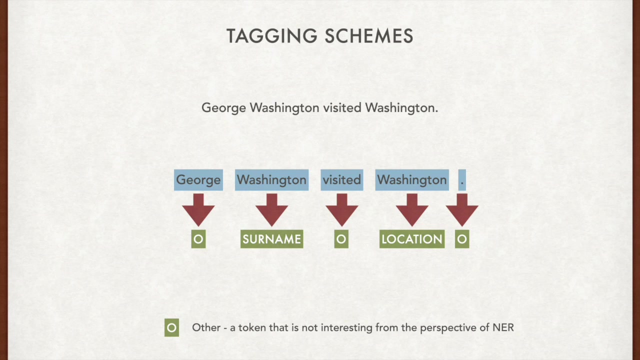 And the idea stressed out by Galibert and Rosset that named entities might span over multiple tokens has some interesting implications that we will discuss in a moment. For now, let's think about how our model can solve the problem. Named entities span over tokens, so, having some input text, let's tokenize it first. 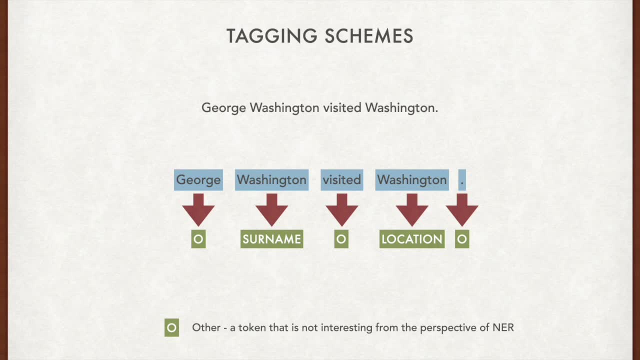 Then we can apply a sequence stacking approach. Assume that we have a tokenized text- George Washington visited Washington period- And a set of labels we want to relate to those tokens. here we have surnames and locations. Our model could classify each token, assigning the label surname to the first Washington's. 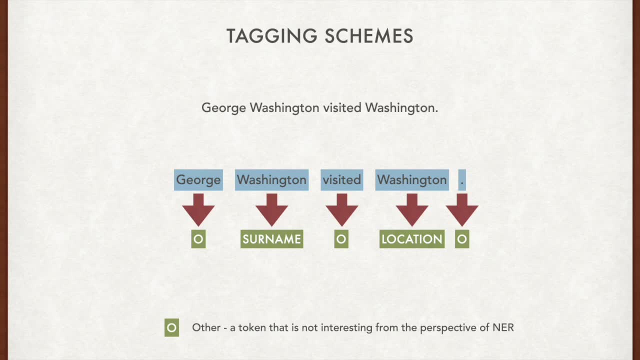 occurrence and the label location to the second one. As we can see, the word Washington is polysemic, So the information about the context is required to assign correct labels. Finally, we can introduce some special label O representing all others uninteresting from. 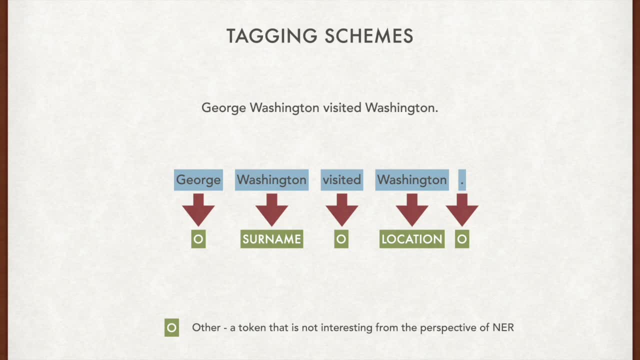 our perspective, tokens that do not form entities. Hence our solution: must assign each token in our sequence one of the labels, ook surname or location. Great, We treat the problem as a token level classification here. but is it enough? Sometimes yes, but in general no. Assigning each token a 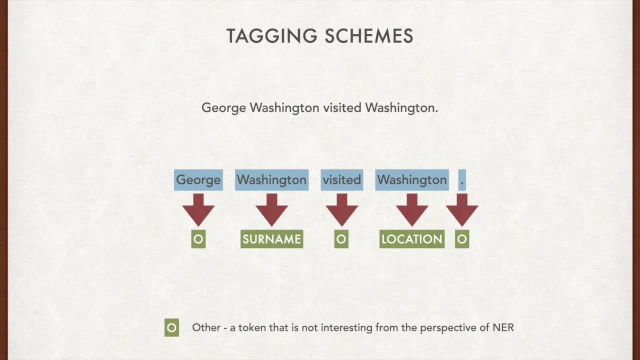 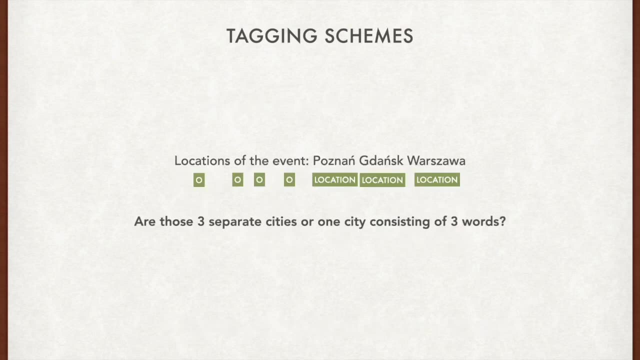 label indicating a category, as presented in this slide, works great until we encounter two challenges: combined Named entities might consist of a sequence of tokens, they might span over multiple tokens and named entities might be located next to each other, as in the example in this slide. Imagine the 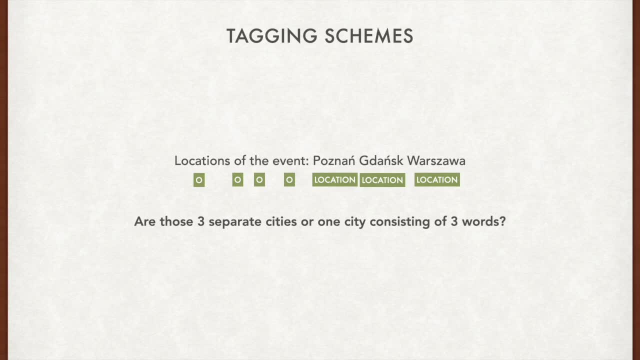 following scenario: We process a tweet in which someone puts three cities next to each other without using commas. There exists some bad people, but we don't have to worry about them. We can just ignore them and let them go. I know several ones. some of them even put spaces before question marks and periods. 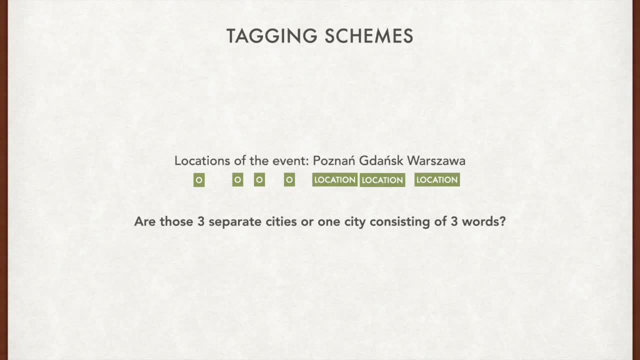 In the following sequence locations of the event: Poznań, Gdańsk, Warszawa. all cities are marked as locations. Great wait, no, How can we decide whether those three tokens represent three separate locations or a single location consisting of three tokens? Or maybe? 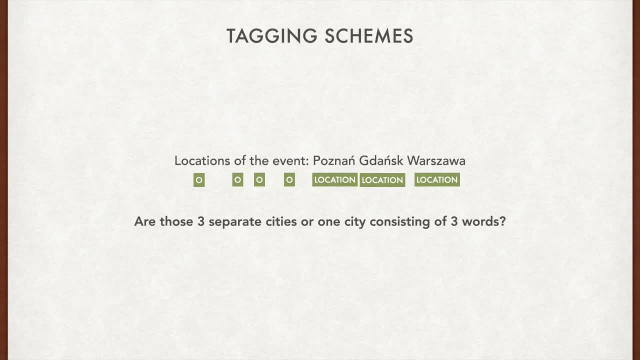 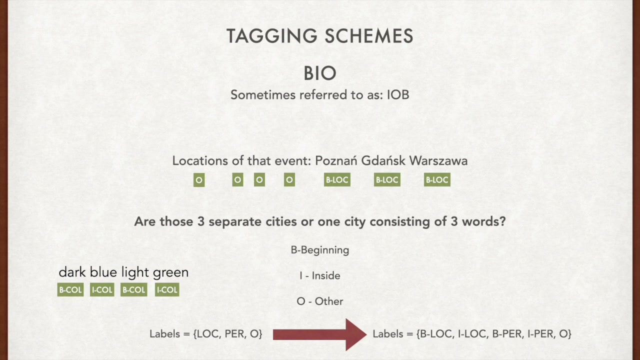 there is some pair of cities where each undecided person soak the prey, We don't know. though it'd be wise to add one unique магical grid which can be used to assign different boundaries to the respective entities. We might enrich the set of our labels using the Bio. 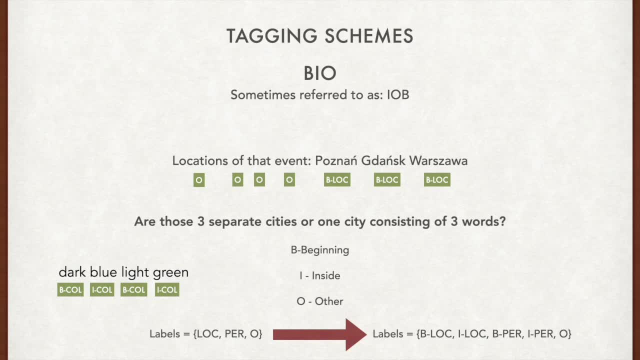 Bio refers to three kinds of entities we might have. O refers to the case already described. O is used to tag all tokens that are not related to any entities entity we want to extract. B refers to the first token in a sequence representing an entity. 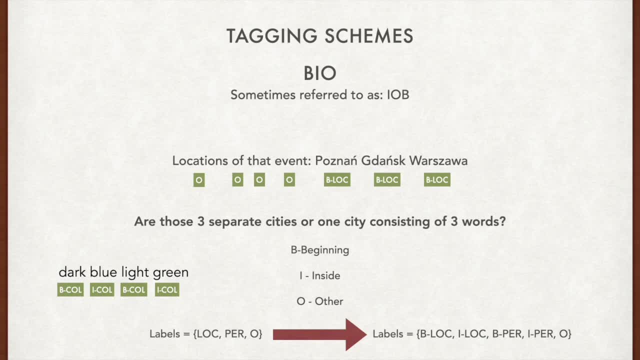 B stands for the beginning of the entity. I refers to all but first tokens in a sequence representing an entity. I stands for the insight and represents the continuation of an entity which started with the token marked as B As our named. entity recognition tasks usually involve multiple categories like location. 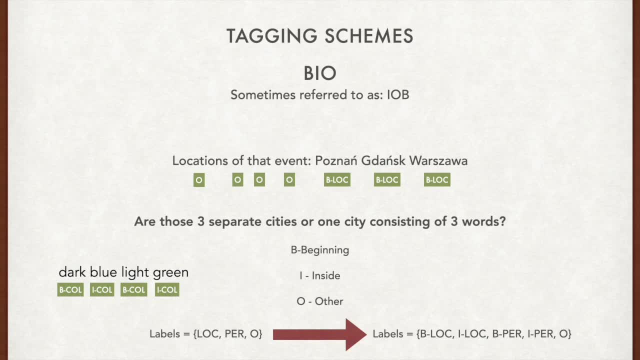 and mentions about people. we should introduce both B beginning and I inside for each entity type defined. As we can see at the bottom of our slide, we add B' and I' prefixes to each category name in our label set. Thus the initial set of possible labels increased from 3 to 5, because now we consider the beginning. 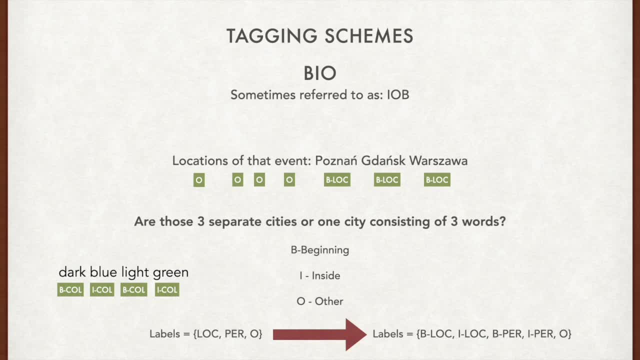 of a location and the inside, the continuation of a location separately, as well as the beginning and the continuation of entities representing persons. To save space on the slides, I've shortened the labels: Per refers to a person, Lock refers to a location. 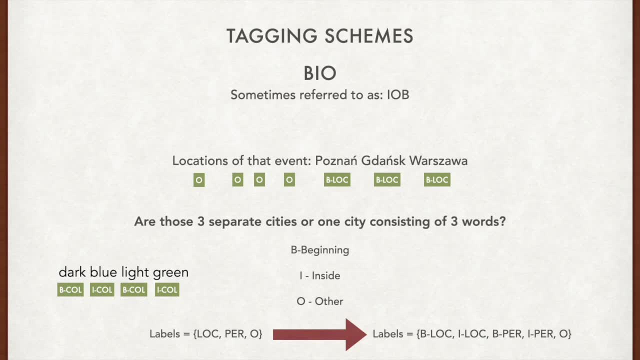 Please note that we don't use prefixes for the O label. As tokens marked as O don't form entities, we don't need to use beginnings and insides in that context. Now we can use those new tags to tag each token again as each of the city names are. 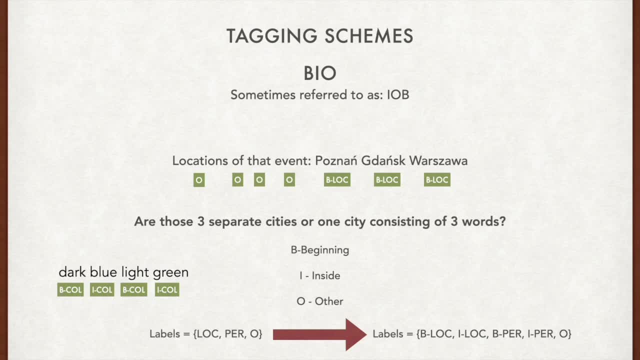 tagged with the BLOCK label, We can see that each token represents a new entity, a different city. Similarly, considering a sample input- dark, blue, light, green- from which we would like to extract entities representing colors, or COL for short, we could use the following: 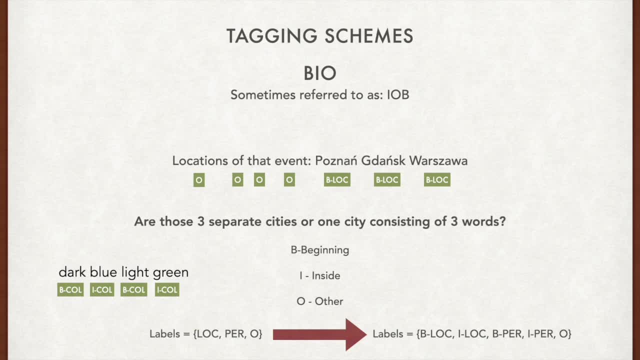 tags to state that the first two tokens- dark blue- represent the first color and the second two tokens represent the first color. Some other color here: light, green. We know this because dark and light are prefixed with the B letter, so that we know that these: 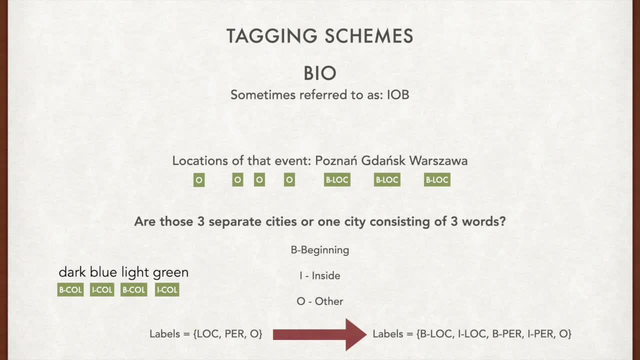 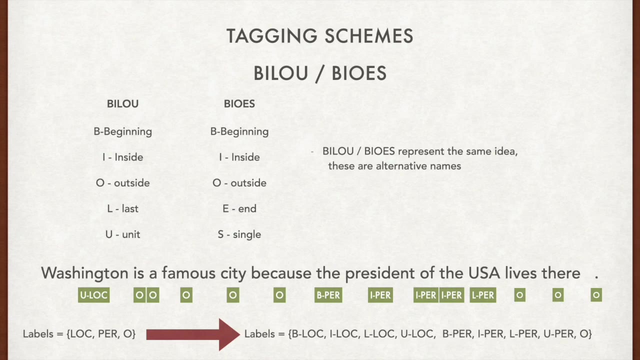 tokens are the beginnings of new entities and because blue and green tokens are marked as continuations of entities started with B. However, some problems might be solved, achieving higher quality, if we use another tagging scheme that is even richer in information. There are two popular schemes that are supersets of the BIO scheme, and both of them refer: 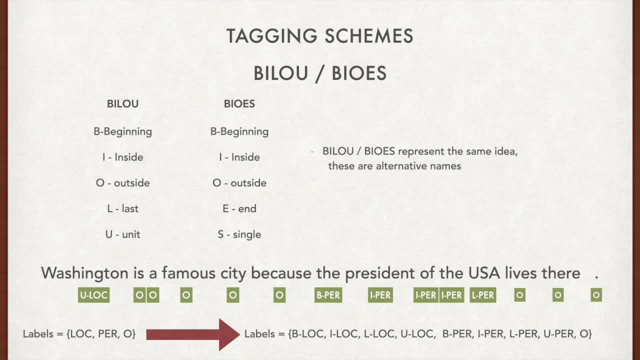 to the same idea using only different names. These tagging schemes are BLOCK and BIOES. In both schemes the BIO part represents the same cases as in the previous slide, but they add some additional prefixes that can be added to our categories. to mark the last token, 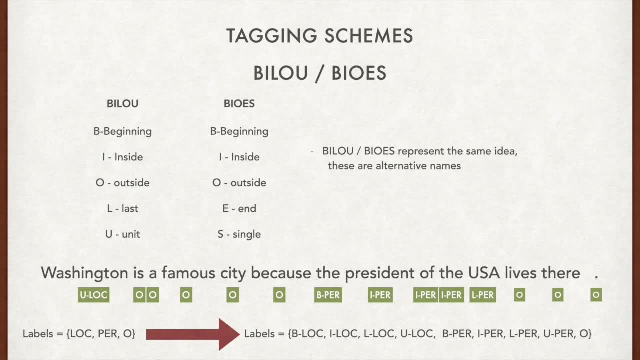 In our entity, We might use the L prefix coming from the BLO and the E prefix coming from the BIOES. L here stands for the last and E stands for the end. both of them are semantically the same. Also, in case when an entity mentioned consists of only one token, the authors of BLO and 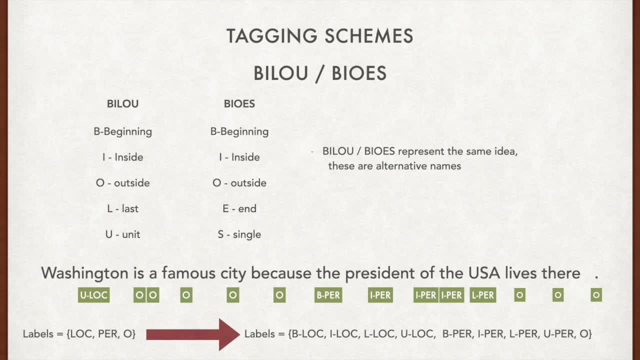 BIOES propose to mark them using a special prefix, U or S, Instead of tagging them using B prefix representing the beginning of an entity consisting of a single token. The U letter in BLO stands for unit and the S letter in BIOES stands for single. 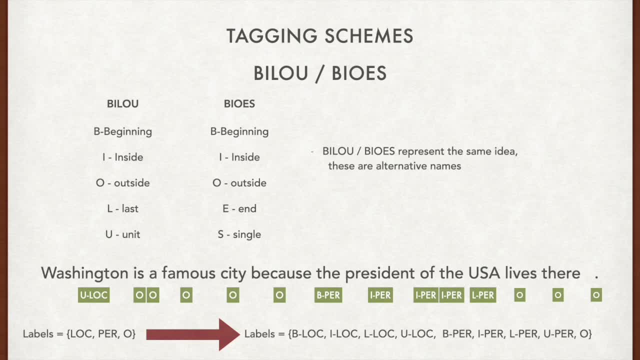 The interpretation of both letters are the same. Sample text tagged using the BLO scheme is shown on this slide. The sequence Washington is a famous city because the President of the USA lives here is tokenized. The first Washington token obtains the ULOG label representing unit location, a location. 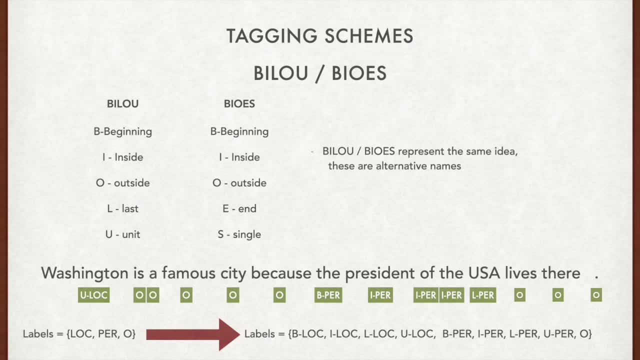 that consists of only one token- Ok, it's here, let's go- of the USA is also tagged. The first token, D, obtains the B person label, which stands for the beginning of an entity representing a person, while the last token, the USA token. 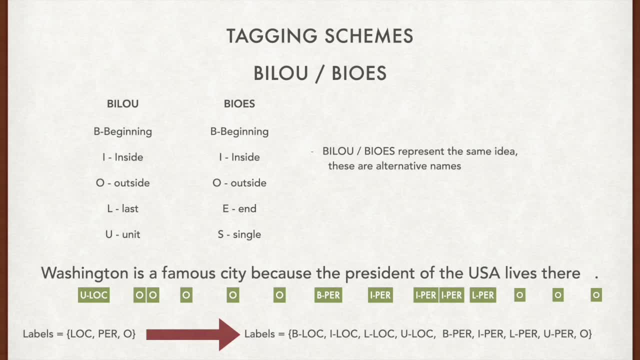 obtains the L person label, which stands for the last token in an entity representing a person, and all other tokens between the beginning and the last token obtain the I person label. as these are the insides of the entity, You might wonder: why would I use these tagging? 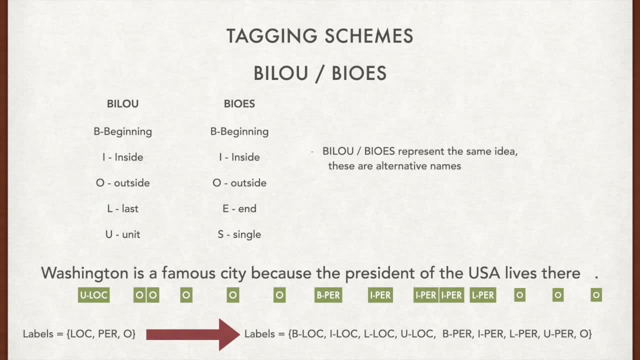 schemes instead of simple bio, And the answer is: it depends on the problem. While the most popular tagging scheme is indeed bio because it is a simpler one, sometimes you use a simple tagging scheme because it is a simpler one. sometimes you use a simple tagging scheme because it is a simpler one. sometimes you 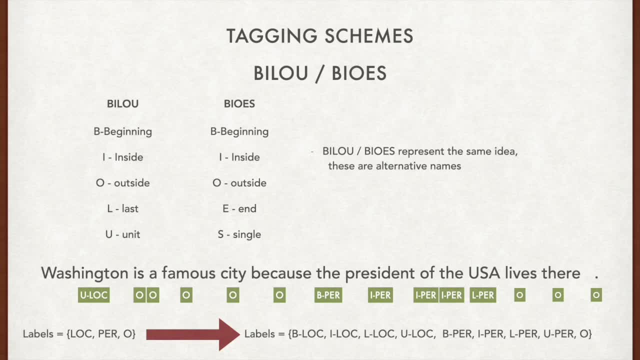 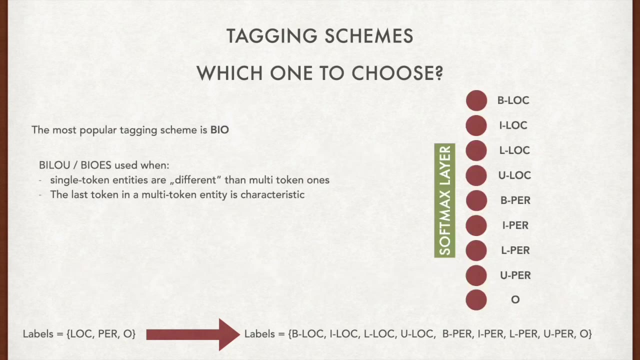 use a simple tagging scheme because it is a simpler one. sometimes you do bilel and the quality increases, but it is still not as good. Usually we need to verify it empirically. by doing some experiments, However, we can assess to some extent whether we might benefit from using Bilel or BioEase. 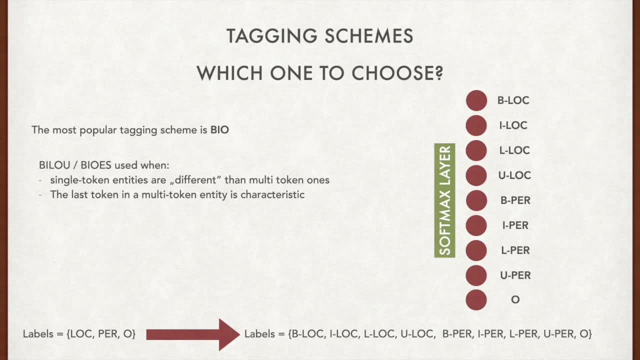 if we keep in mind how those prefixes help us solve problems Today. neural networks are ubiquitous the world of natural language processing, so they also dominated the named entity recognition task. We can imagine a neural network that assigns one of the predefined labels based 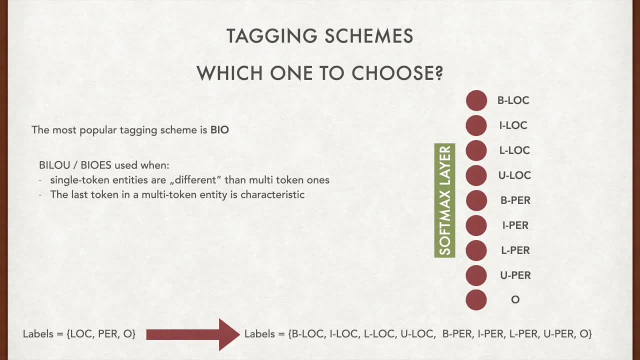 on the output of some softmax activated layer, like the one presented here in the slide. For each possible label we have exactly one output neuron assigned. If a given token represents, for example, the beginning of a location, the first neuron should output the highest probability. 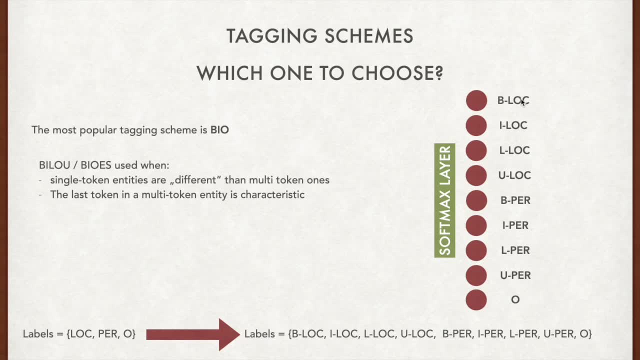 This slide shows us that each output neuron specializes. each of them tries to detect and the label it is assigned. We might consider utilizing below or by OE stagging schemes. In all cases, we might consider using BELOW or BYOE stagging schemes. In all cases, we 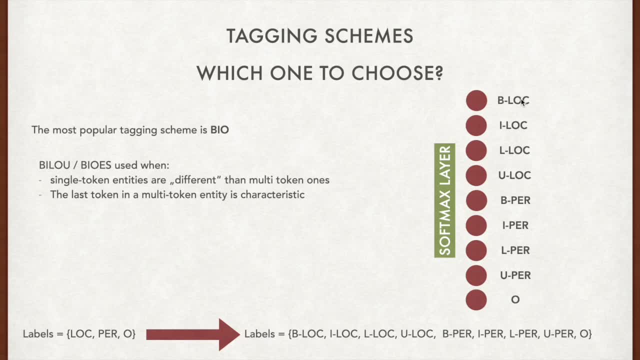 might consider using BELOW or BYOE stagging schemes. In all cases, we might consider using single token entities. If there is some specific quality that makes single token entities characteristic, maybe it is worth introducing a separate neuron learning to detect only such cases. Similarly, 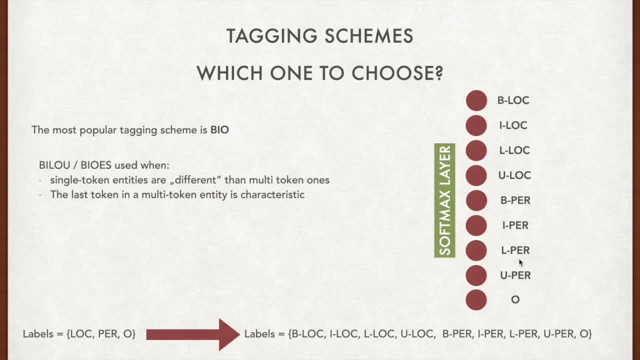 if we have some specific quality- not just a single case, but a separate entity. there is a possibility to measure the value of a single token entity and use it to determine quality. that makes our last tokens in multi-token entities special and different from other tokens that are a continuation of an entity. maybe it is worth introducing a separate token. 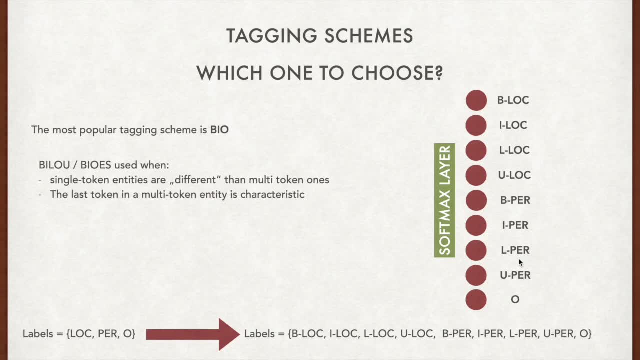 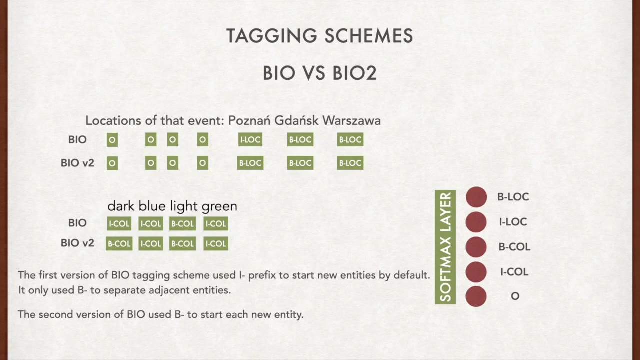 a separate neuron, learning to detect only such cases To be maximally precise. for historical reasons, there are two versions of the BIOS scheme, alternatively referred to as IOB scheme. The scheme we described in the previous slides is the newer version 2, which is frequently referred to simply as the BIOS scheme. To 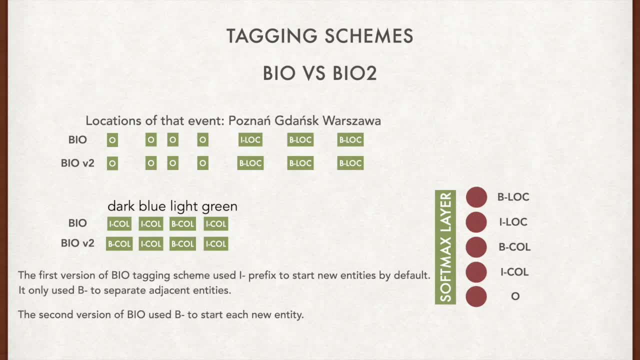 avoid confusion, it is always preferable to specify whether we use the original BIOS or BIO version 2.. The historical BIO scheme differed only in one aspect: The B prefix wasn't used at the beginning of every new entity. Instead, the B prefix was used only for those entity. 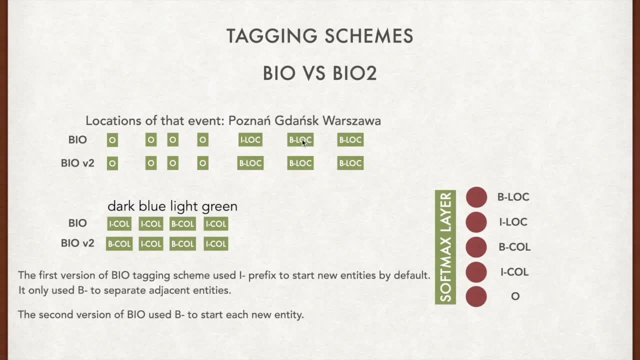 starting tokens which were preceded by another entity of the same type. Otherwise, we used the I prefixed token to start a given entity, As we can see in this slide in the original BIO scheme, if before a given entity there is no other entity of the same type but there is, for instance, the beginning of the sequence. 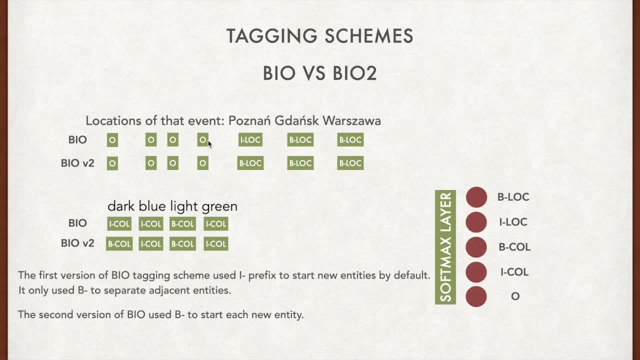 or a token marked as O. we use the ILOC and ICOLE labels, even if they represent first tokens in another, the ILOC and ICOLE labels, even if they represent first tokens in another an entity. The b-prefix was reserved only for those situations where we needed to mark 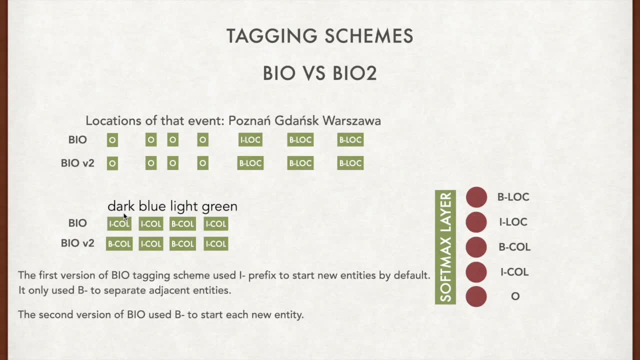 that a given token marks a new entity. otherwise we would generate ambiguity. we already discussed, However, from the perspective of neurons in the output layer of the neural network. this old BIO tagging scheme introduced some representation inconsistency: The same beginning of a given entity, for example place, would sometimes be marked as bplace and sometimes iplace. 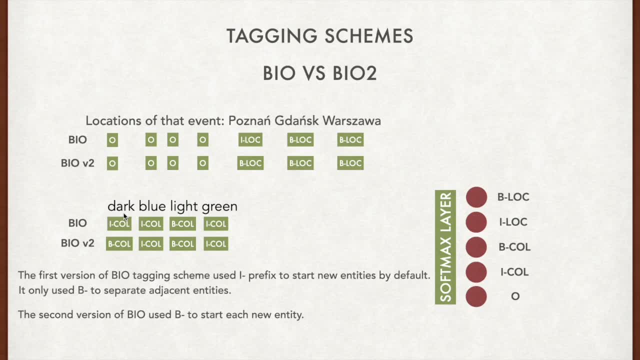 depending on the previous labels, of the previous tokens in a sequence. For this reason, many people start each new entity with b using the BIO v2 tagging scheme and frequently it's the default. Now, as we described the problem, we know how the output can be generated. we know that. 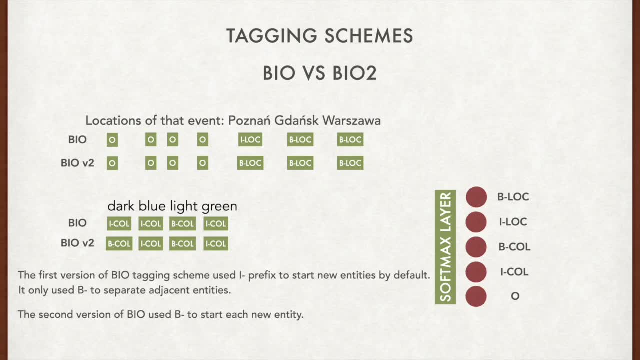 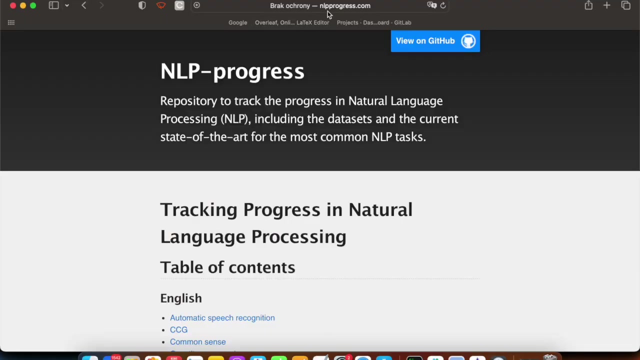 the training set might consist of pairs of a given token and the expected label prefixed. using the BIO scheme, we might discuss some of the most popular architectures used to solve named entity recognition tasks. The website called nlpprogresscom collects the list of the most popular tasks in natural 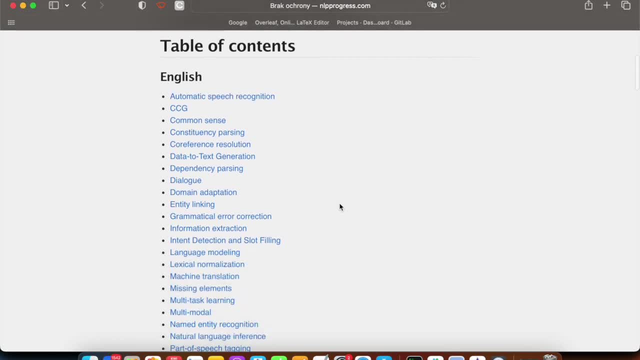 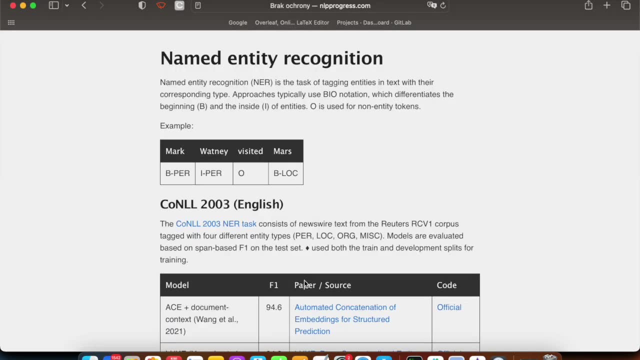 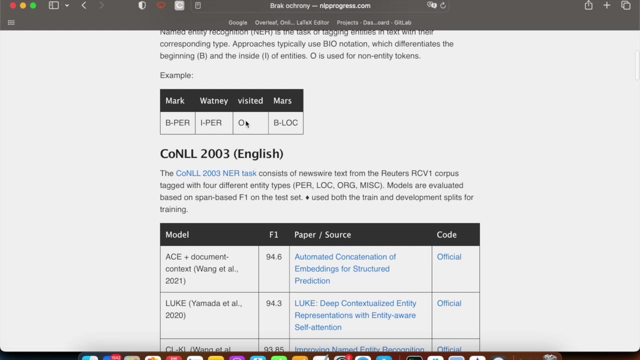 language processing, among which we have the named entity recognition task. If we click here, we obtain a ranking of solutions per a given dataset: TIP 3. NLP- Progresscom. 3. NLP- Progresscom. 4. NLP- Progresscom. 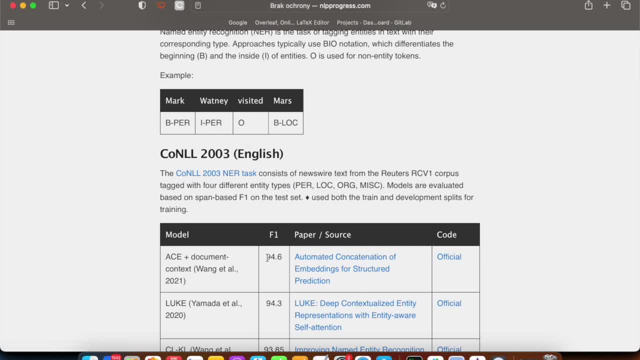 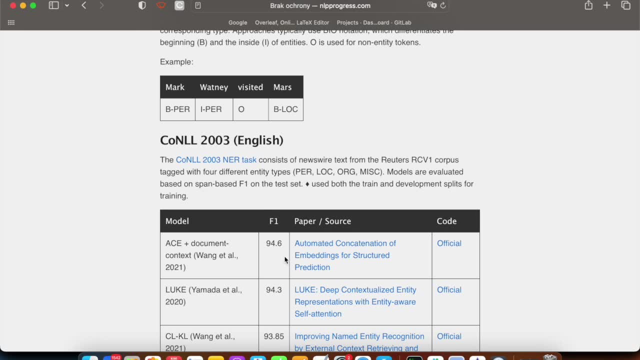 5. NLP Progresscom. 6. NLP Progresscom. 7. NLP Progresscom. 8. NLP Progresscom, 9. NLP Progresscom, 10. NLP Progresscom. 10.. solutions are ranked according to some selected quality measure. Here it is F1 score. 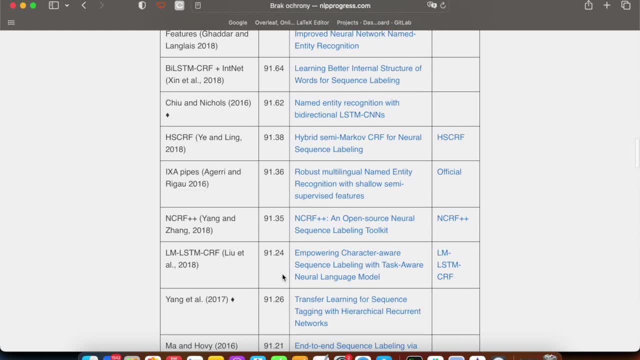 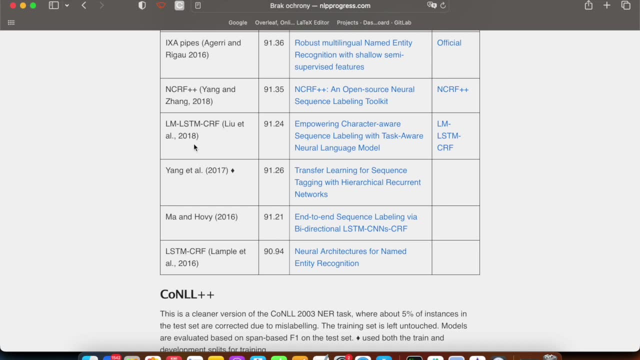 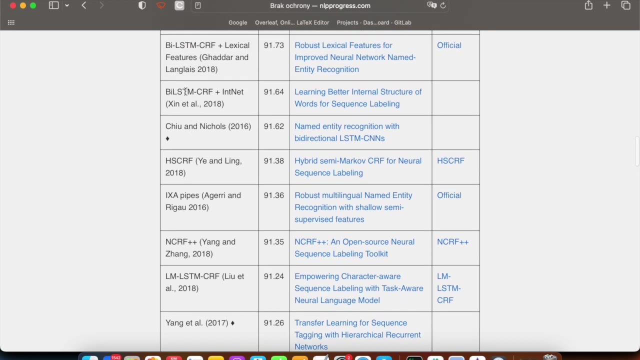 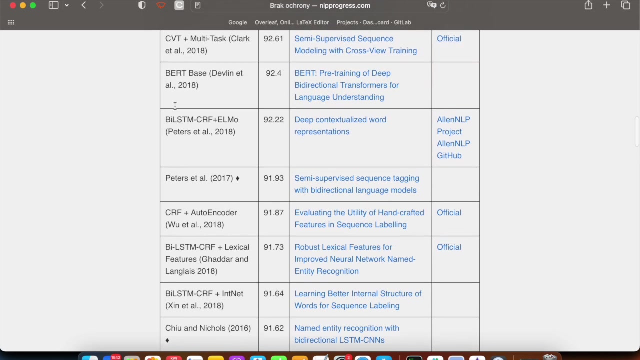 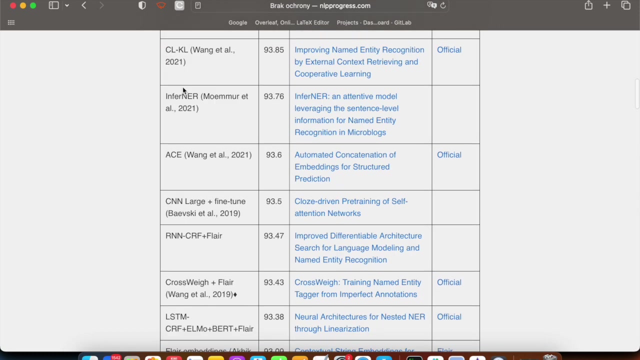 As we can see in the list provided, there are some approaches that recur frequently, Like the LSTM layer, which is here and here, and also here we have ByLSTM, next ByLSTM. this is ELMO, which is based on LSTMs, LSTM, more LSTM- yeah. 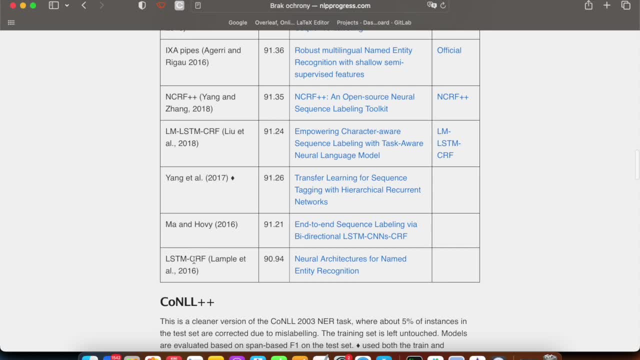 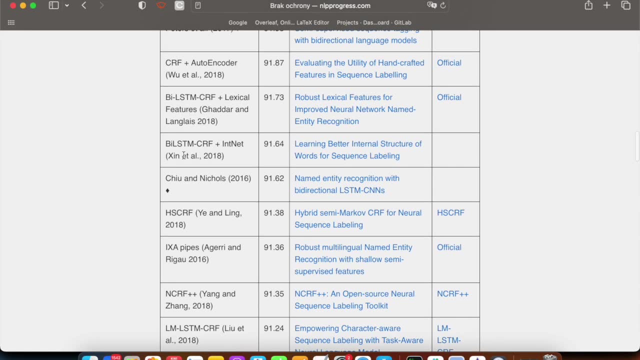 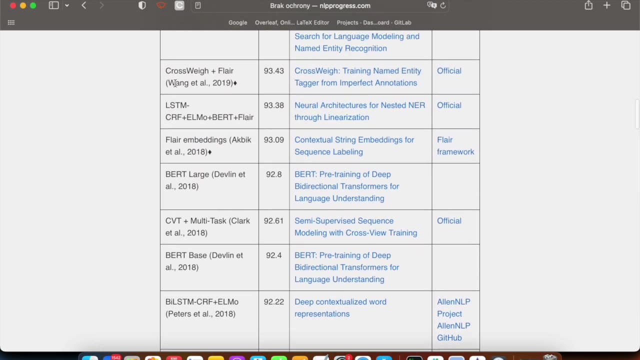 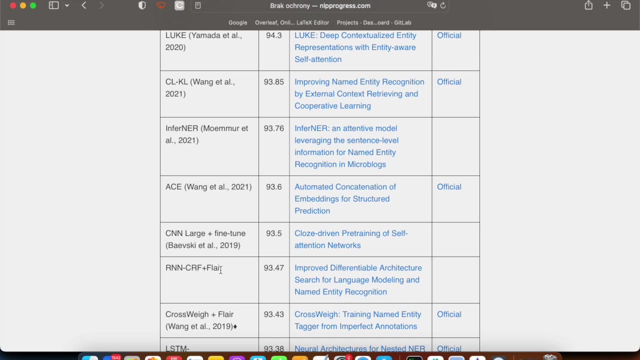 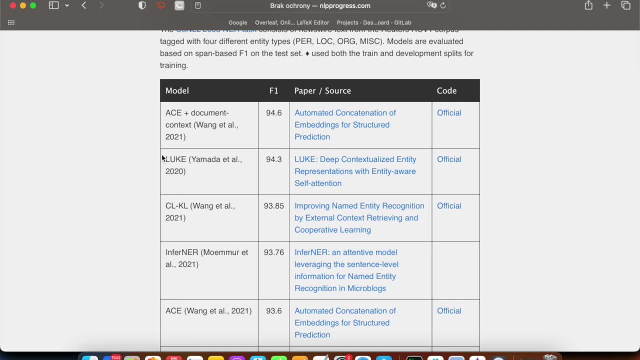 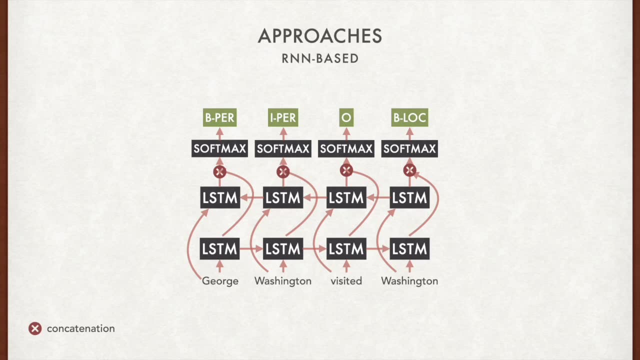 look. Now let's analyze how some of those methods work. A straightforward solution that can come to our mind after the lecture describing contextual embeddings from recurrent neural networks is to use a bi-directional LSTM model that utilizes some number of LSTM cells- reading the text in a left-to-right manner, and some 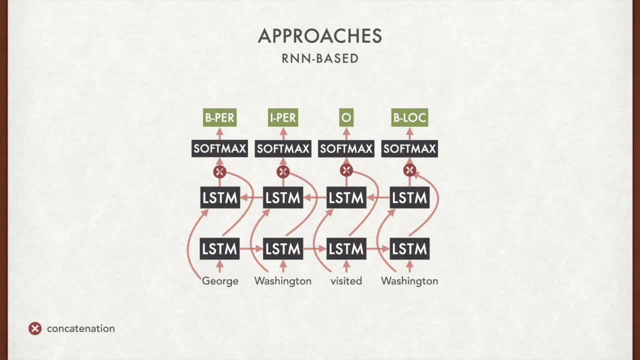 number of LSTM cells reading the text in a right-to-left manner. Here we have one example. Here we have one example. Here we have one left-to-right LSTM layer and one right-to-left LSTM layer. That network generates context-aware representations of tokens. 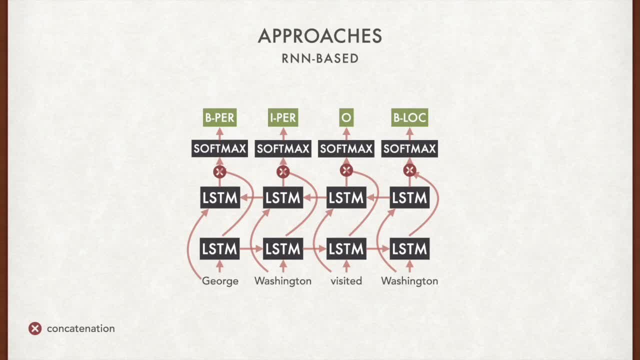 Both LSTM cells obtain the static embeddings assigned to input words and generate context-aware embeddings, One embedding of a given word which is aware of, for instance, in the case of the word visited. the output of the LSTM: Okay. The left-to-right LSTM layer is a representation aware of everything that was read so far in. 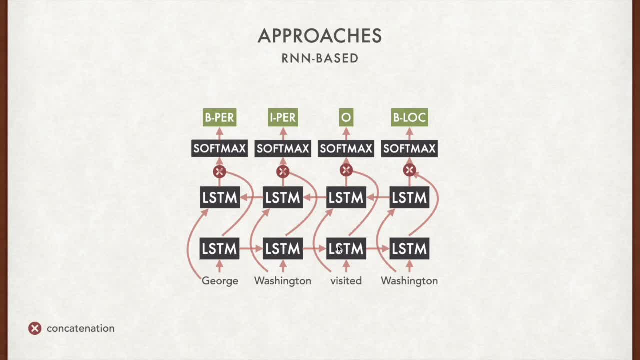 that sequence and the right-to-left reading LSTM layer generates another representation of the same word, but the representation that is aware of everything that is put later in that sequence. Okay, So that this representation of the word visited is aware of the left-to-right LSTM layer and. 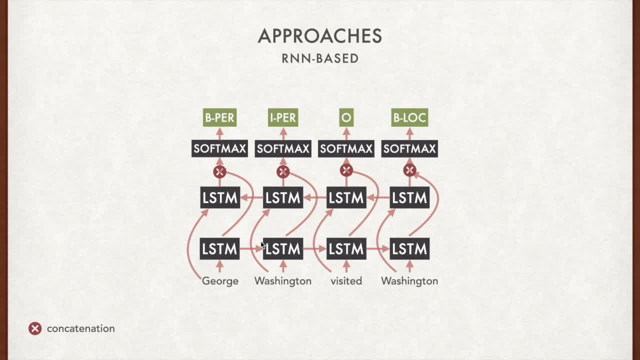 we can then write it in one right-to-left reading LSTM layer. Okay, hand side context: George Washington visited and this LSTM cell is aware of, in the context of the word visited, is aware of the of the next token, the token Washington. Then we use the concatenation. 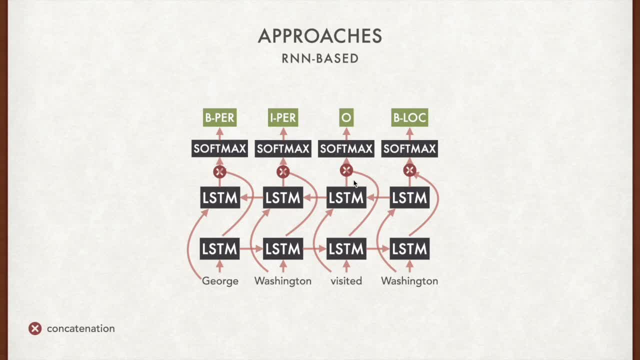 procedure to join those embeddings generated in the hidden states of those LSTM layers and process it through the softmax layer so that we can classify each token according to our label set. This way, the second, Washington, can be classified as a location because the embedding generated here is aware that the previous token was visited, so probably we visit some. 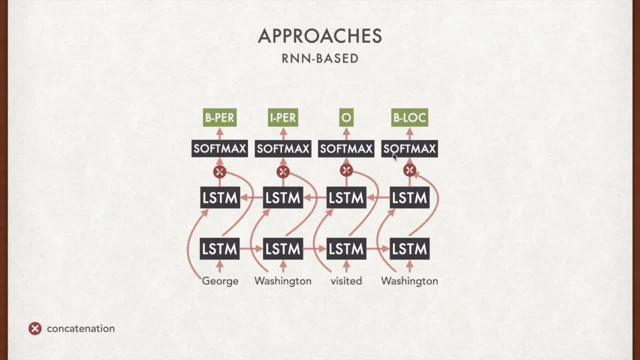 location. That's why it can generate the label stating that Washington is a location. Similarly, Washington, related to the second token, is classified as a continuation of a person because previously we saw that the previous word is George- Probably some name, and Washington is likely to be the surname of that of that person. 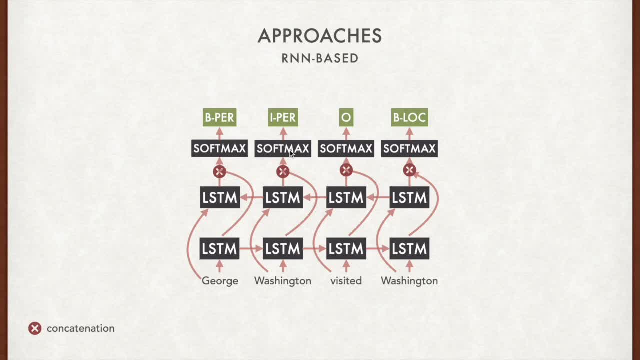 And this approach was the most popular one in the pre-transformer era, and some variations on using bi-directional LSTM layers are still successful, as many top solutions listed on NLP progress contained LSTM in their names. There are even multiple improvements that can be applied. 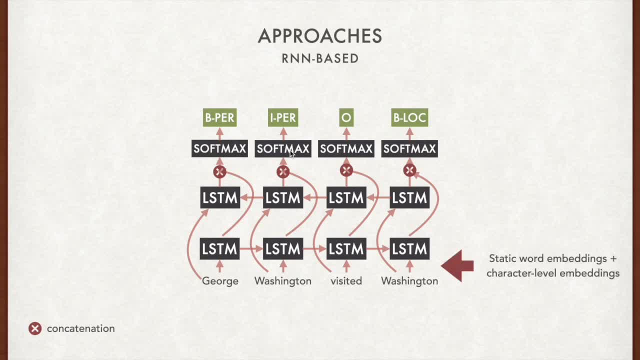 let's now take a look at a complete representation. icted So this will work, But was it possible to rewrite this solution around the connection or function? Eastern and Eastern connection may work too, but sometimes none. support of neural networks is made勝 zinc. 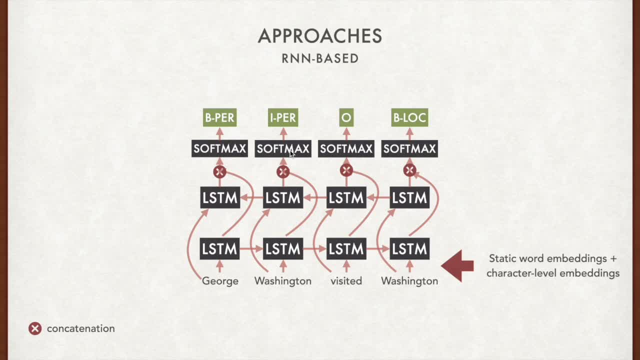 Structure level embeddings is to generate embeddings based on how words are constructed and to prevent a situation in which static word level embedding cannot be constructed Because if a given word we process was not observed during the training, we don't know how to map that never observed token to a static embedding. 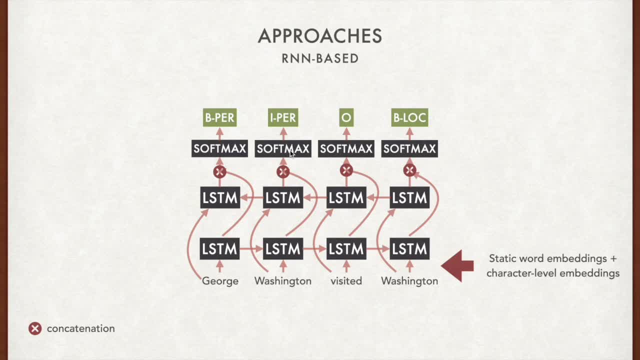 For example, when you use Glove and we have a map of words related to vectors And if we notice some new word that we don't know, it's not possible to generate a meaningful vector for this. However, as character level embeddings construct embeddings based on characters, we can always 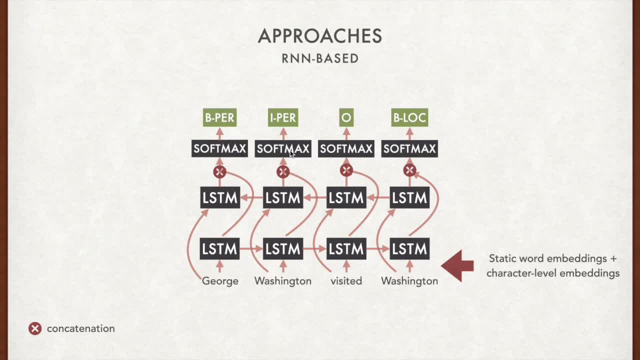 produce the representation so that, even if a given word was not observed, at least the portion of information we can create is not observed. We can always produce the representation so that, even if a given word was not observed, produced by these character-level embeddings, will be meaningful. 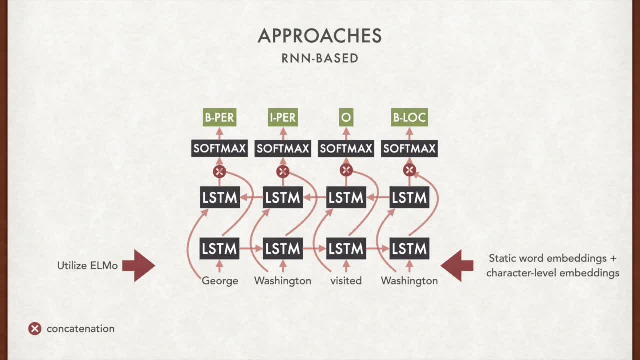 Subsequently, we can also inject representations coming from ELMo. As we might remember from the third lecture on contextual word embeddings based on recurrent neural networks, ELMo was trained using a language model objective so that it learns some general-purpose representations of words. These can be: 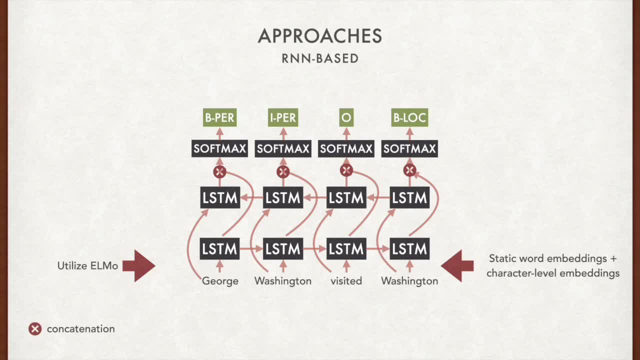 injected to our solution to enrich the representations we have in our network. Since these are context-aware embeddings representing the meaning of words, we can use ELMo as an external frozen feature representation provider and for each token processed, we inject information from ELMo into our pipelins, For example, in the same way as in the: 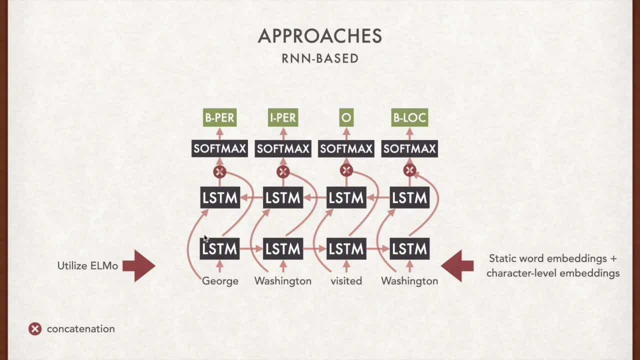 original instruction exercise. original ELMO paper. by concatenating the ELMO vector assigned to a given word with a contextual embedding constructed as the output of the first LSTM layer. If you would like to understand this idea in detail, please watch the third lecture recording available in our course. 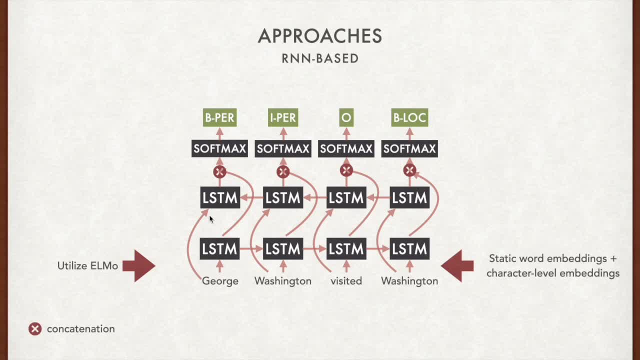 Finally, some successful applications integrate with the CRF algorithm, which stands for conditional random fields. The theory behind CRF is quite complex and math-heavy, so here I would like to provide you with some general overview of the idea and, if you are interested in. 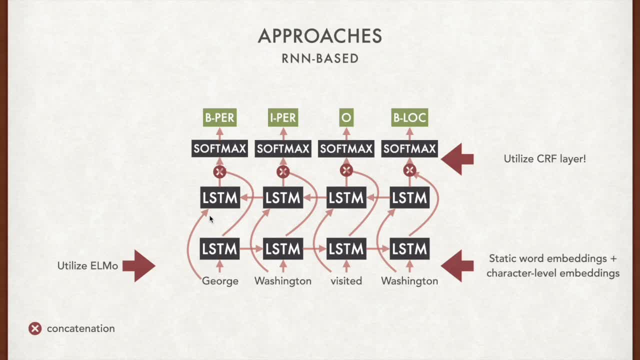 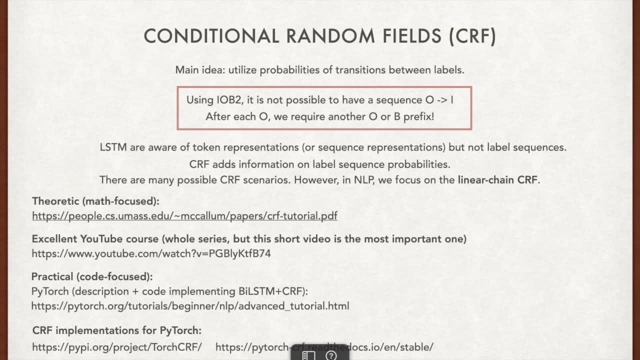 the details, I attach some good materials describing the topic. The CRF algorithm can be used for sequence classification and the most important aspect of it, fact that it not only uses features describing a given element in a sequence, for example the embedding assigned to the given token, but it also models probabilities of sequences. 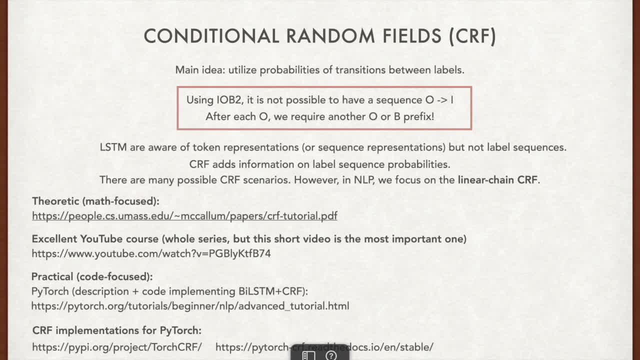 of labels. What does it mean In named entity recognition task? some sequences of labels are likely and others should be prohibited. If a given token, let's say the token visited, is assigned with the O label, the next token, Washington representing a city, has to be: 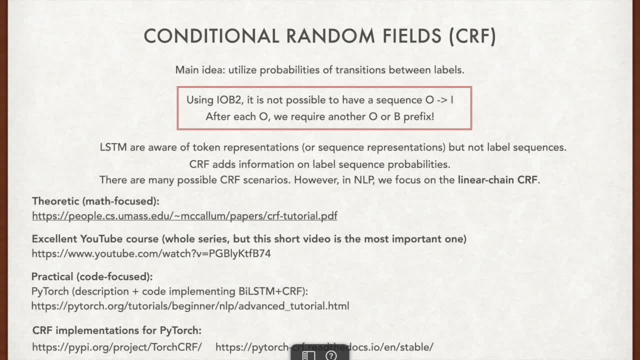 assuming bio-tagging scheme prefixed with B. It cannot be prefixed with I because the beginning of each sequence has to be marked with B. We cannot tell that the first token in the entity is the continuation, And this is something that CRF or conditional random. 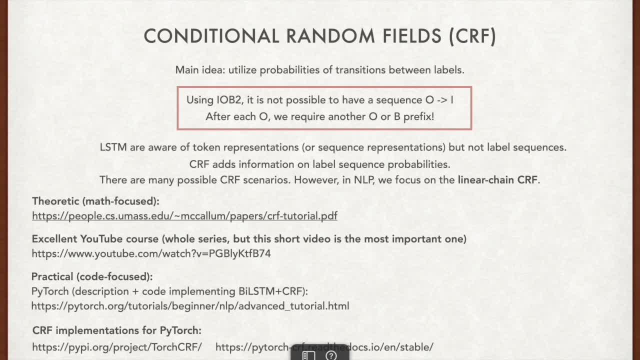 field because the CRF is an abbreviation. this is something that conditional random fields allow us to focus on. If we think about a regular LSTM cell, it only focuses on features describing tokens modeling the sequence in the LSTM-hidden cell. To make predictions, they use that hidden state and process it through some classification. 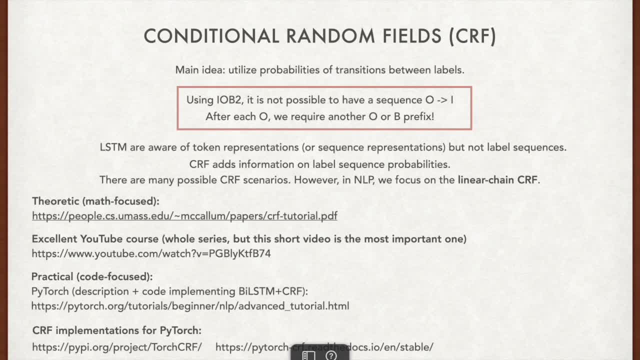 layer, So it doesn't use the information about the sequence of labels explicitly. So joining it with conditional random fields allows us not only to look at those features describing tokens, but also check which sequences of labels are the most probable ones. Fortunately, in the world of neural networks, conditional 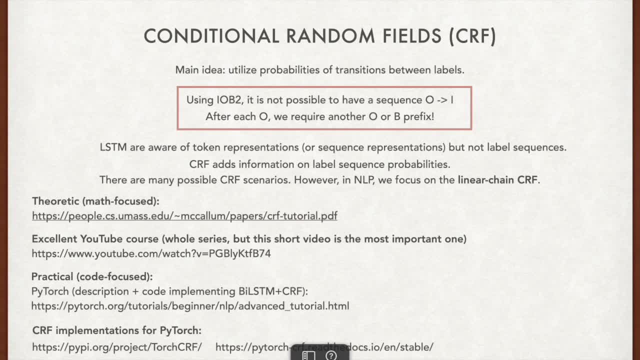 random fields can be implemented as a single layer used in the network and there are several attempts to create a library integrating with PyTorch so that we can simply import that layer and use it in our code. At the bottom of this slide you can find some links to libraries implementing CRF conditional. 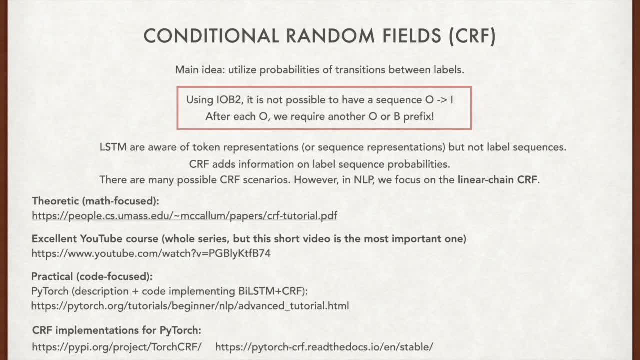 random fields As a PyTorch layer. One of the best exhausting descriptions of conditional random fields is provided by Charles Sutton and Andrew McCallum, where Andrew McCallum was one of the inventors of this idea. You can find a link to the tutorial here in the slide. however, be aware it's long, 35 pages. 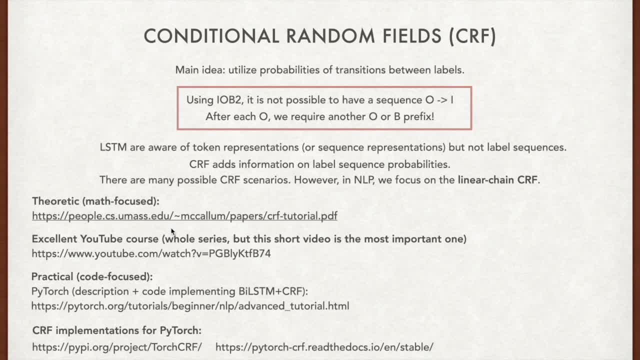 long and math heavy. Fortunately, in the context of natural language processing, we mostly focus on a specific class of conditional random fields, called linear chain conditional random fields. If you prefer videos Hugo La Rochelle, the lead of the Google Brain team in Montreal. 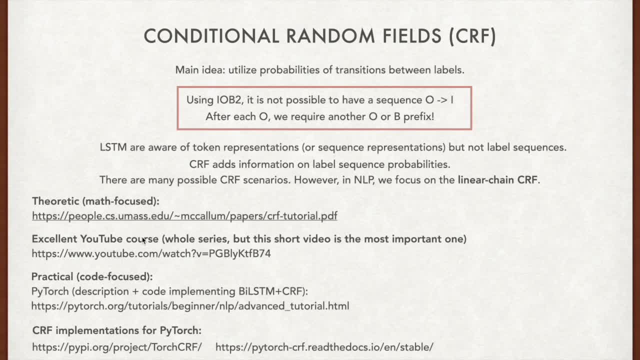 and an adjunct professor at a university in Montreal, gave a great series of short lectures on conditional random fields that is available on YouTube. The video linked in this slide is the second one in the series. It's short- it's about 8 minutes long- and describes the idea very intuitively. 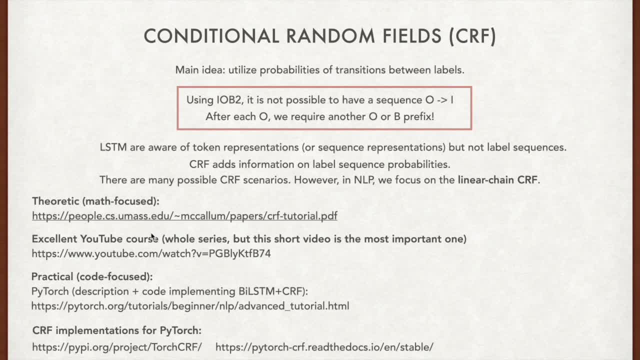 Finally, if you prefer, looking at some code, there is a great tutorial on how to code conditional random fields in PyTorch and integrate it with LSTMs. A link to that tutorial is also provided here in the slide. Looking at the ranking of solutions, it seems that it's always worse to add conditional 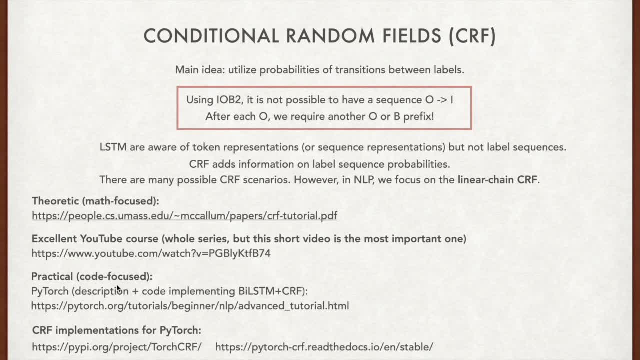 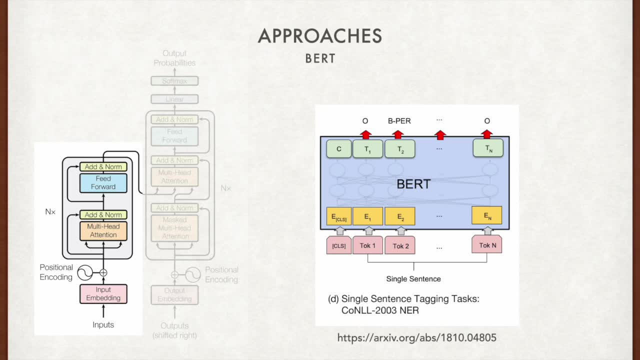 random fields layer. when using LSTM networks for named entity recognition, An alternative family of solution is based on the BERT model instead of LSTM. We focused on BERT during the last lecture. To shortly summarize this approach, we used the Transformers Encoder to embed each token in our SQL. 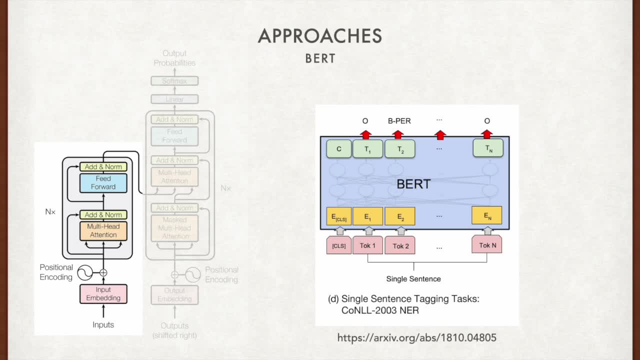 You can find an example of this in the description below. I hope you enjoyed this video. If you liked it, please leave a like and share it with your friends. If you don't, you can also subscribe to our channel. Thank you for your support. 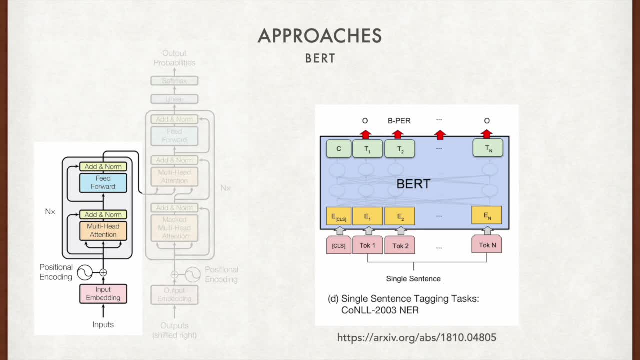 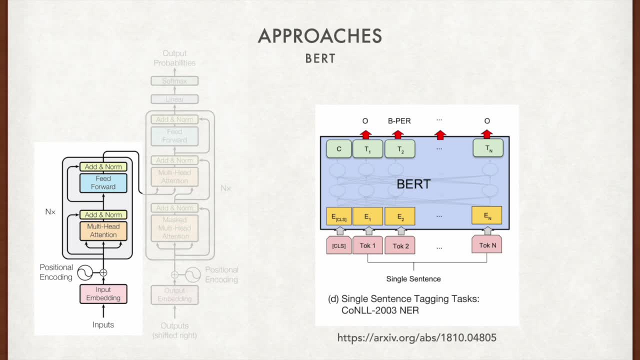 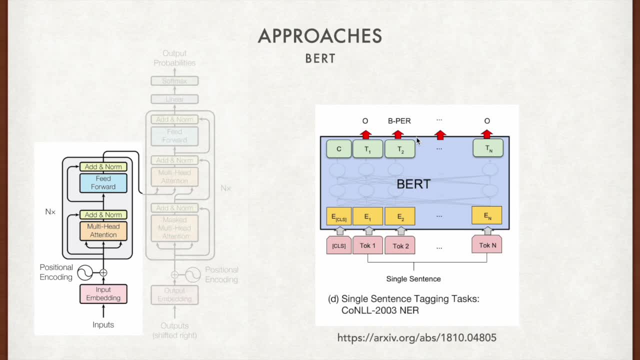 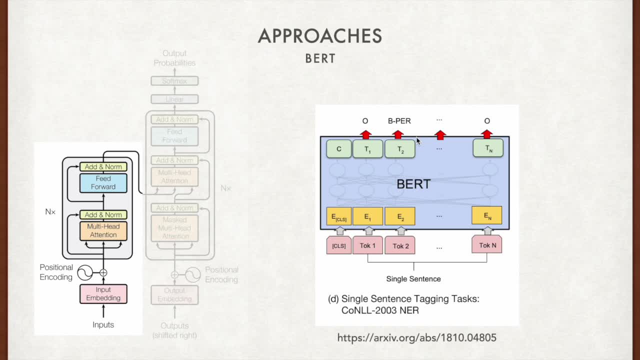 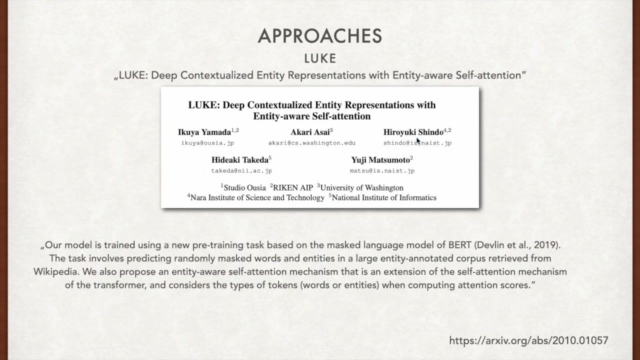 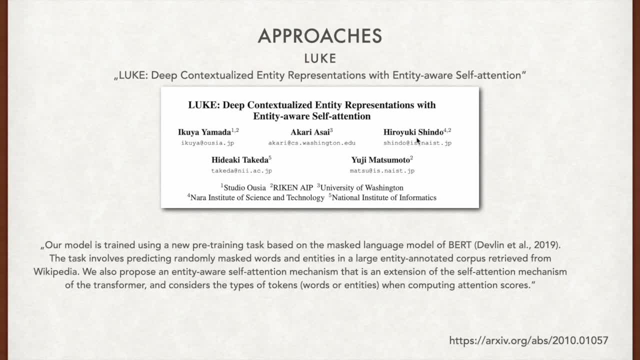 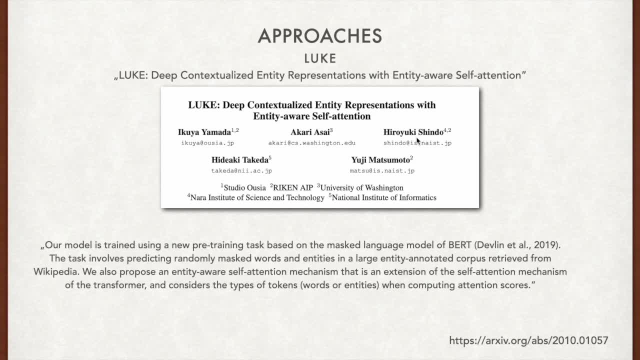 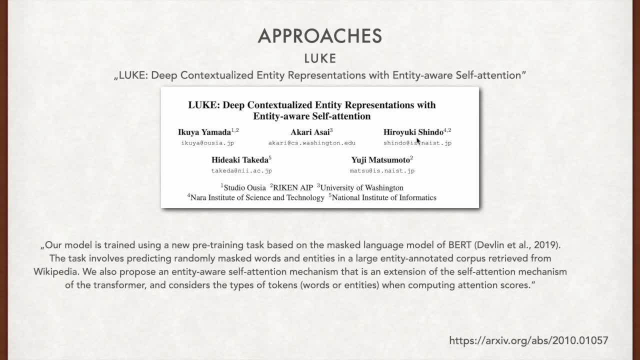 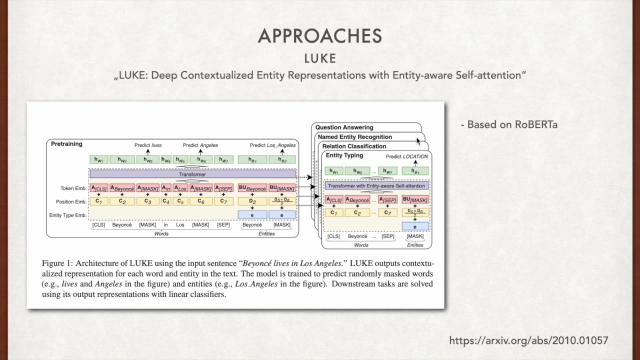 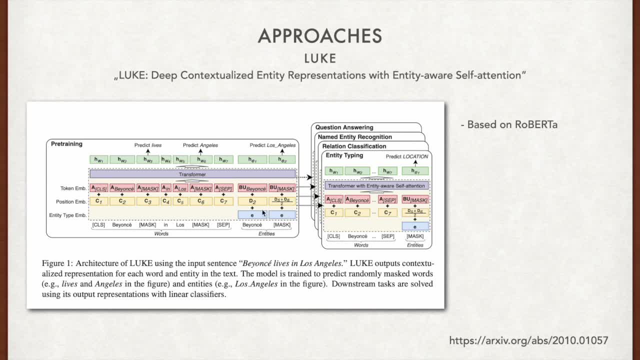 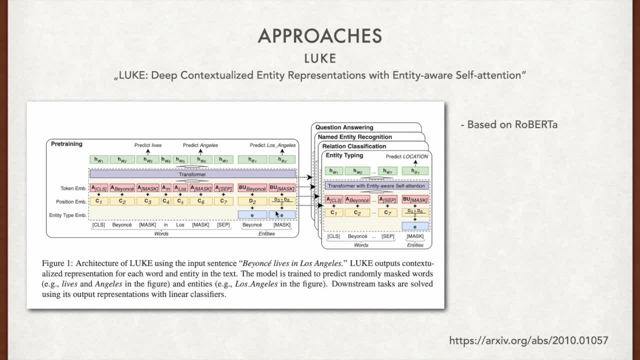 to the representations of entities only. As we have two kinds of inputs to the network- regular tokens here and entities separated using the SEP token- the authors decided to introduce a modification to the calculations of the self-attention scores. We already discussed it in the context of transformers that there are several ways. 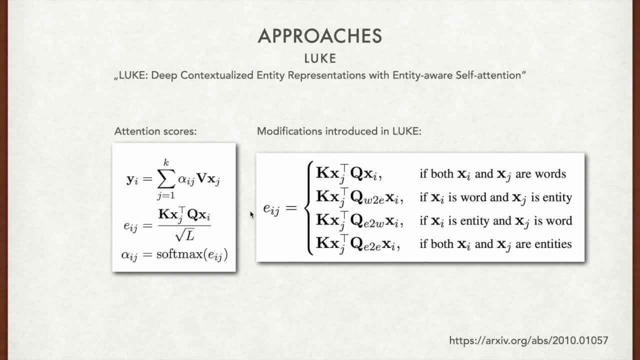 of calculating similarity between vectors. So far we used the dot product to calculate the similarity between keys and queries in the attention mechanism, but the authors utilized several possible transformations. depending on the situation, We used different transformations. if both elements compared, are words Ok. 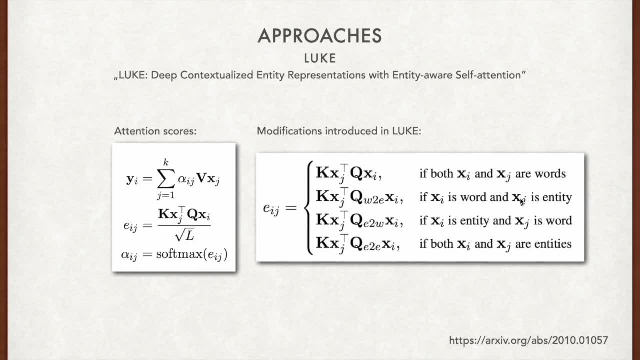 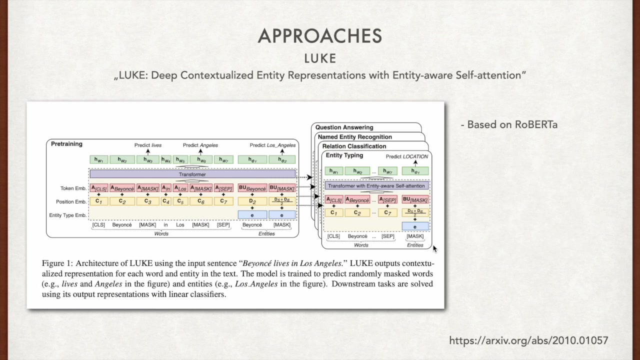 Different when only one of them is a word and the other is entity, and these situations are not symmetric, And a different one if both of them are entities. This way, the network learns relations between words and entities better. When applying the pre-trained network to the named entity recognition task, they need to 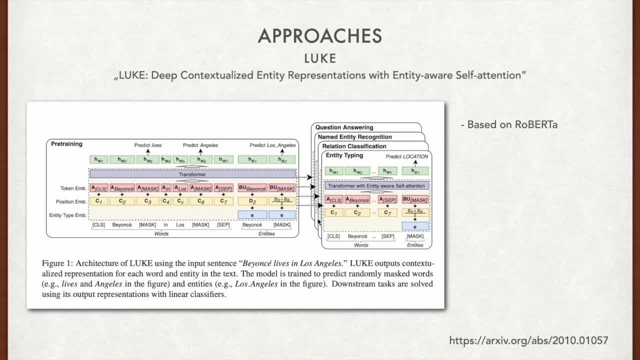 provide some candidates in the entity system In the entities section. But when using the model at the inference time we search for those entities. Our goal is to find where those entities are. So to solve them they use exhaustive search. They verify each possible n-gram and try to classify it. 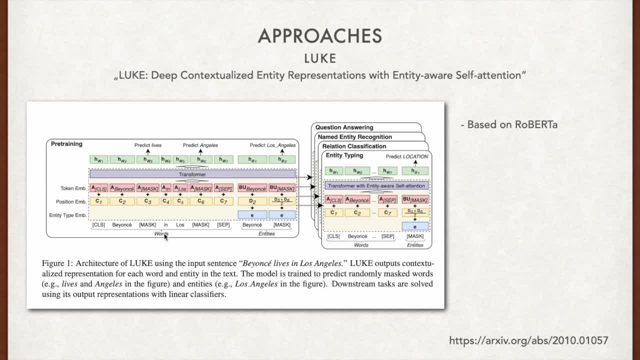 So it might be time consuming. Ok, Let's see how it works. First, we generate a given input sequence, We generate all possible n-grams and then verify whether a given n-gram represents an entity and then try to classify that entity, whether it is a person, a location or something. 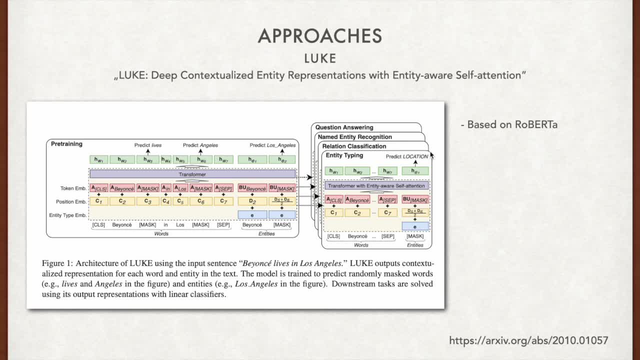 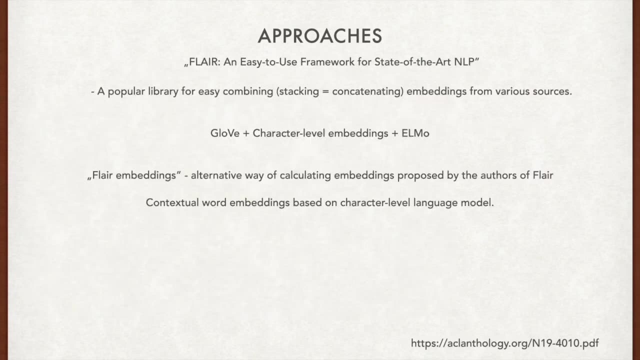 different or something that is not an entity, And the look model is the second best approach. today It's ranked second in the nlpprogresscom website. Ok, Let's see how it works. Yet another very popular alternative that produces great results is Flare. 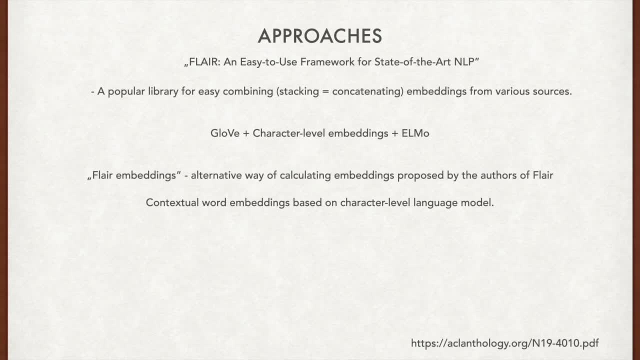 In general, Flare is an NLP framework which allows us to solve various NLP tasks, combining various types of embeddings easily. For example, it allows us to concatenate or stack, as the authors called it, Glove embeddings, Word2Vec embeddings and ELMO embeddings. 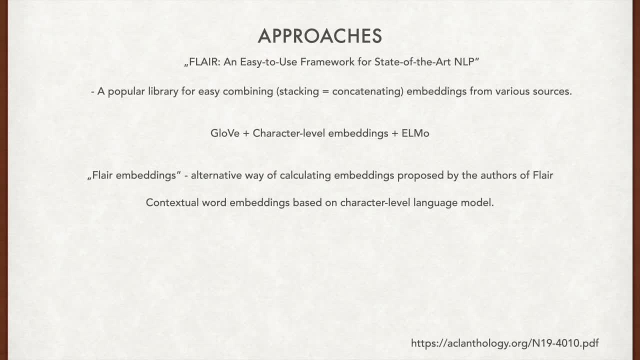 Ok, But from the perspective of our lecture it's more important that the authors of Flare propose their own method of generating representations useful in the context of named entity recognition problem In the paper entitled Contextual String Embeddings for Sequence Labeling the authors of Flare. 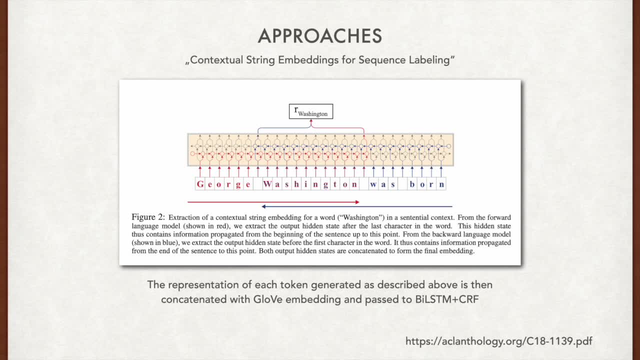 propose to train a bidirectional language model that works on characters rather than whole tokens. That means that the left-to-right language model that consumes a sample input sequence, GEO should be able to predict that in the sequence the next character should be probably R. Similarly, the right-to-left model consumes characters in a reverse order. 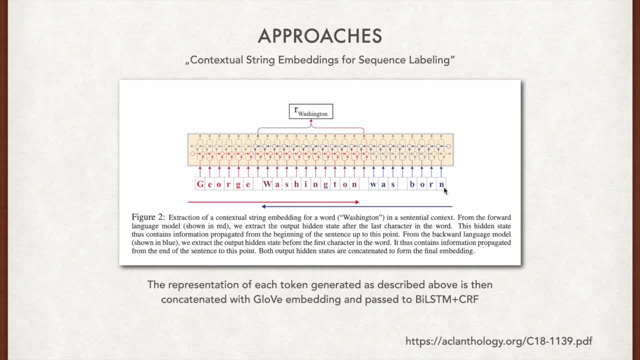 So it should be able to predict that before the characters N and R, the previous one should be O. Those language models are based on LSTM cells so we can extract the embedding representing the whole sequence read so far after reading a given character. Then they used those language models to generate embeddings. 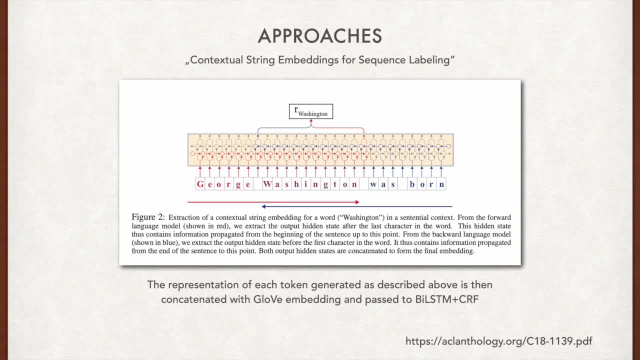 For a given token, for instance the token Washington presented here. they used both language models to construct a single embedding representing this word. They used the hidden state of the LSTM cell generated after reading the whole word Washington. So if we have a left-to-right language model, we process all those characters here. 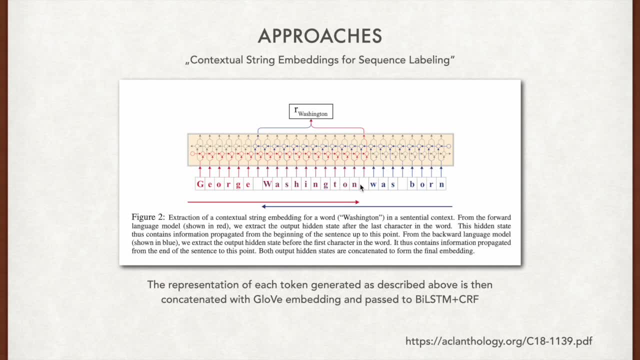 Then we process the last character N and obtain the clone's embedding which will be used to construct the embedding of the whole word. Similarly, they used the output of the right-to-left model so that in the context of Washington, the state recorded, after processing the first character C's and quotient's less than 해. 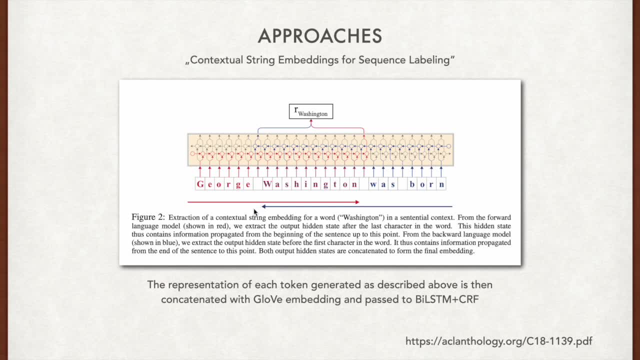 situation is also pick upable in Deb, Portuguese character is also extracted. This is a vector, an embedding, which represents the meaning of that word, Washington, in the context of everything that is put later here in this string. And to produce the representation of the word they propose to concatenate those. 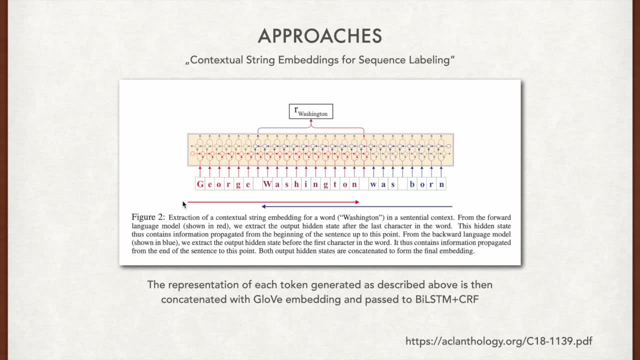 vectors. So first we have a vector that have read the whole sequence, character after character, and we extract the hidden state. after reading n, here We have some embedding and we concatenate it with the embedding produced by the second language model which processes our sequence. 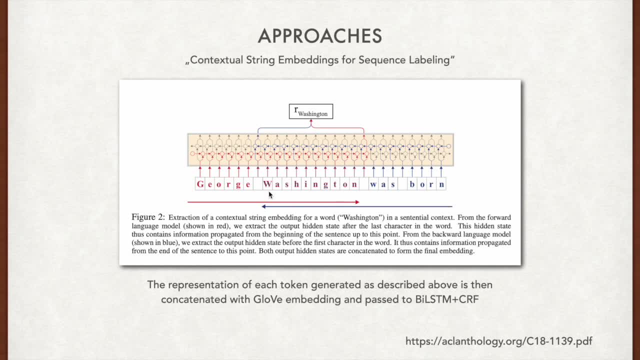 right to left and the output generated before reading, after reading the character w, but from right to left perspective, is also extracted and also used to produce the embedding of the form. So if we concatenate those two representations, we assume that we have an embedding representing. 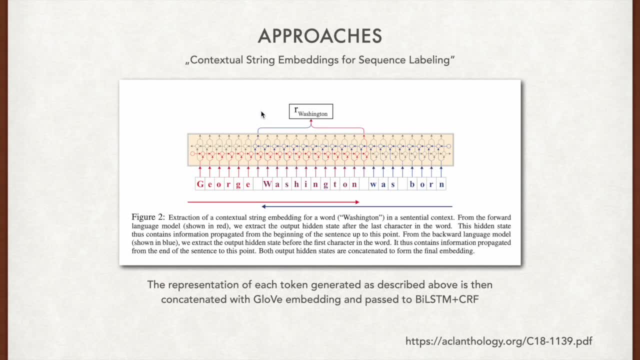 a given word, Here the word Washington. This way we construct word embeddings and now we can move to processing tokens. instead of single characters, because we construct representations of whole tokens, The authors of the paper suggest that it might be possible to use the word Washington to. 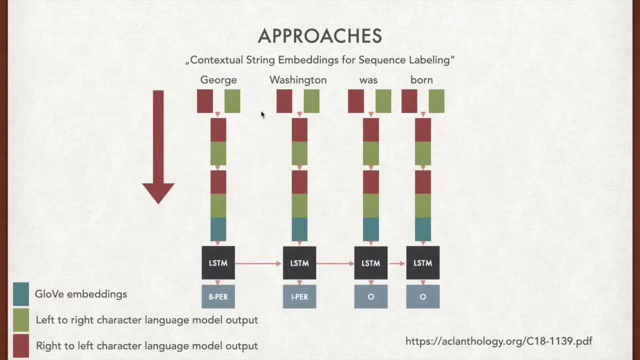 further concatenate these representations with GloVe embeddings so that each token is represented using both character-level embeddings and GloVe vectors, And it's a similar situation to some already discussed solutions where we joined those two embedding types. These concatenated representations are then fed to another BLSTM layer. 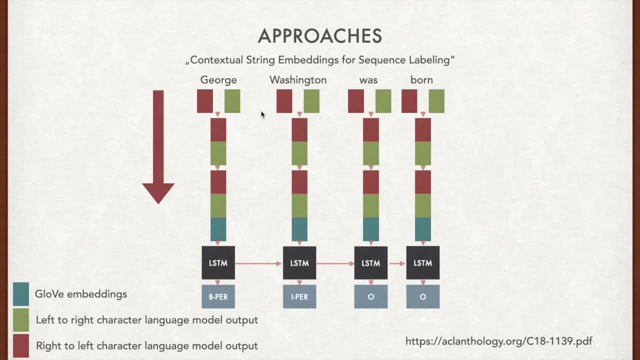 working on those representations and final output of the hidden state is classified tokens Here. because we have limited space, we draw only the left to right BLSTM cell, but there should be another BLSTM layer which reads the same sequence right to left. 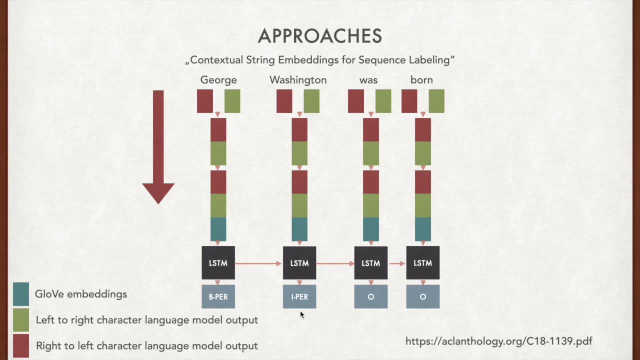 And finally, the output of this should be used to alternate and decide whether a given token represents the beginning of a person or person or the continuation of the person, etc. Those rectangles- red, green and blue- represent various representations, various embeddings. The red one represents the right to left character. 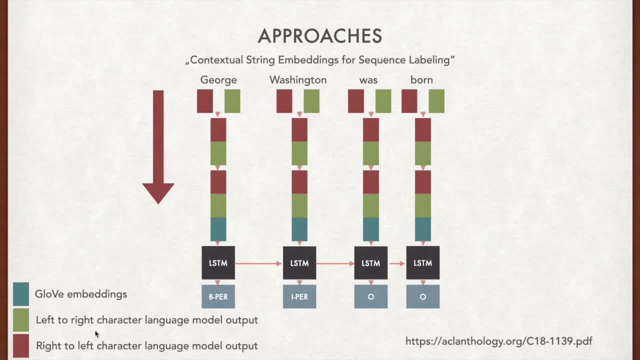 language model output. left to right. character language model output is related to the green one and the blue ones relate to globe embeddings. We join all of them and process it through bidirectional LSTM layers, So here we should have at least two LSTM layers. 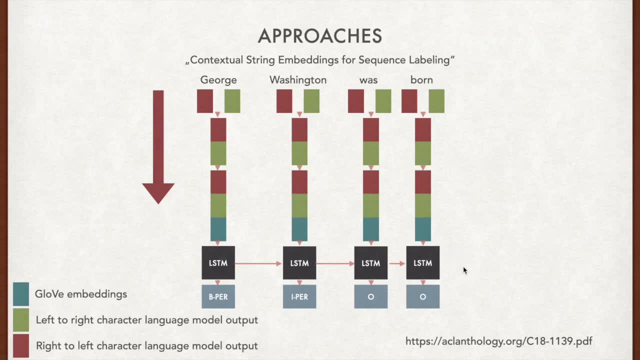 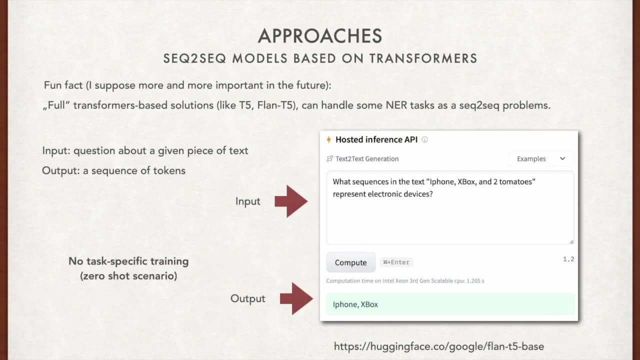 one that reads left to right and one that reads the text right to left. All the methods we described so far involved training, a named entity recognition model based on some training set provided. However, recent advances in natural language processing may even extract some popular named entities without training. We call such a 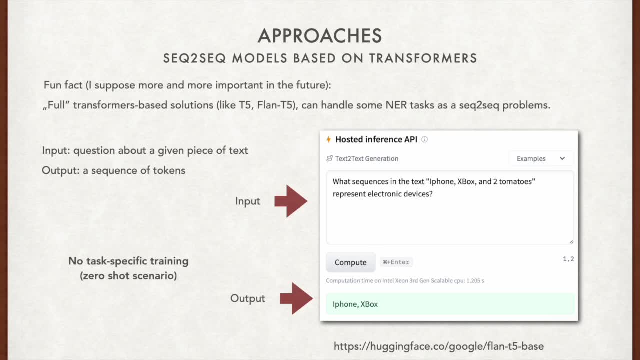 scenario: zero-shot learning. Of course, the quality of such approaches will be worse than specialized models, but we could use those general purpose models and fine-tune them to solve named entity recognition tasks better. The first of the models handling zero-shot scenarios is already known to us. The FLAMM T5 model was trained to transform one sequence. 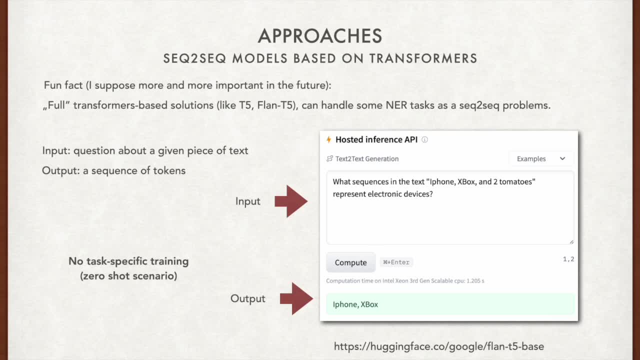 of text into another where the training examples were various tasks to be solved, about 2000 tasks. This way the FLAMM T5 model learned to answer a question machine click and a double-click as the first task. One question that is left asking is: why is the MLSEM used? and one of the하는? 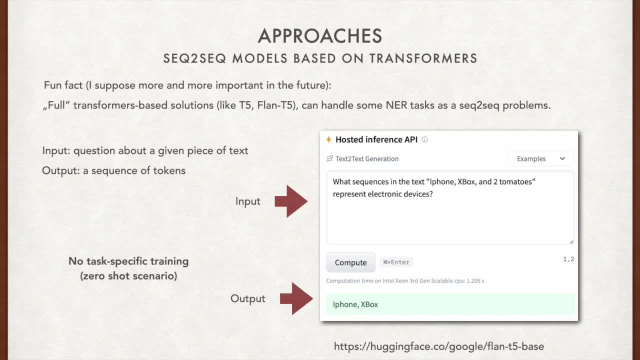 model was trained on almost 2000 tasks. it is highly unlikely that extracting electronic devices was one of the tasks on which the model was trained on, And this is something amazing. but, as we have stated a moment ago, the quality of such solution 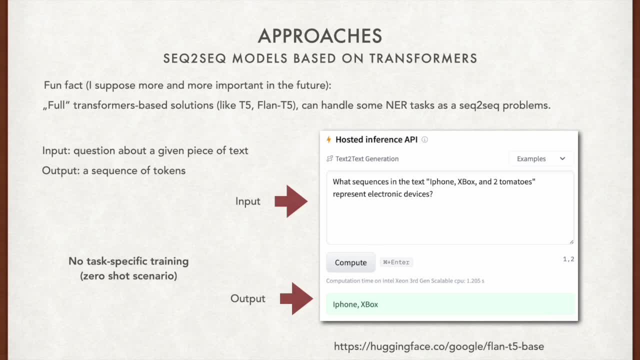 will be probably much worse than the solution specialized to solve only N22 recognition related to that given entity type. However, who knows what the future will bring. Similarly, we can ask ChatGPT to solve the same task. Here it produced a longer piece. 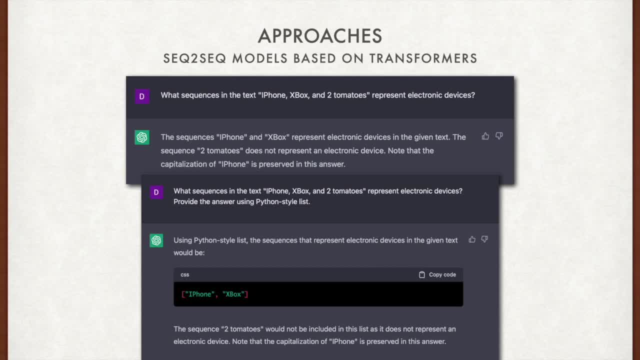 of text that included the expected answer. We can, however, modify the input so that we obtain a list of entities formatted in Python code. As a side note, the comments of ChatGPT about the capitalized code are not the only ones that are not relevant to the solution. 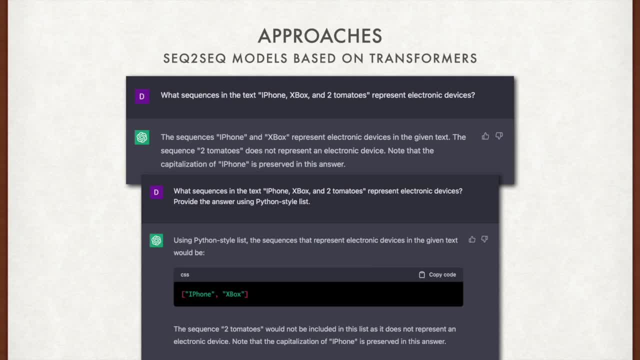 The comments of ChatGPT about the capitalized code are not the only ones that are not relevant to the solution. The comments of ChatGPT about the capitalized code are not the only ones that are not relevant to the solution. We can now see that the capitalization of iPhone might be due to a mistake I made in 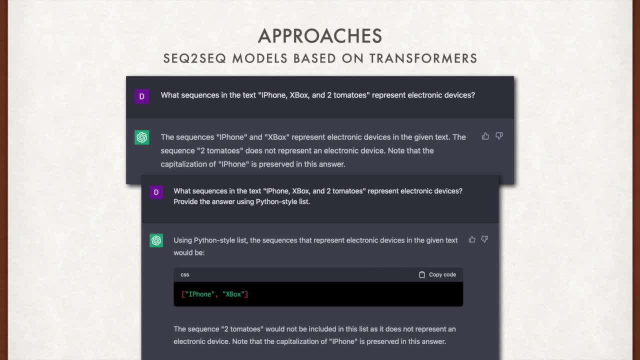 the previous part of the conversation with ChatGPT. First I asked the model to do the same. however, I used lowercase p in the iPhone name. Then I realized that mistake and asked the model to do the same, but this time I used 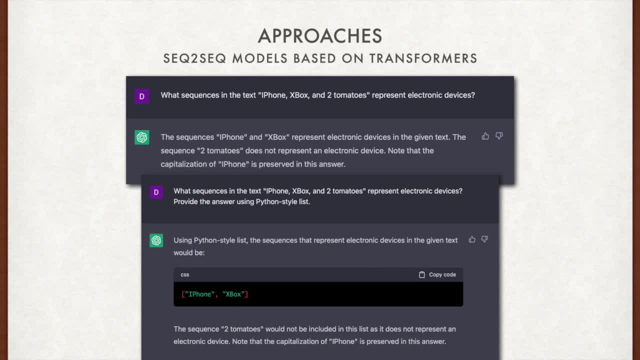 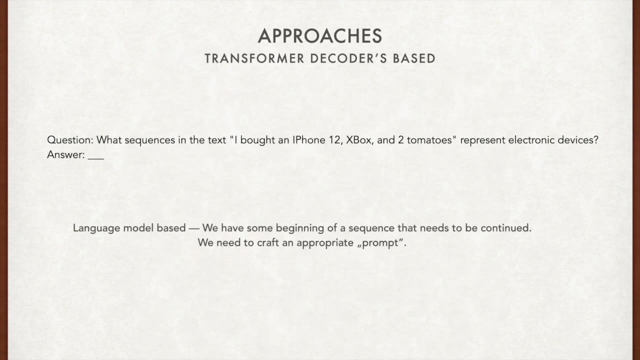 capitalized p letter. The model realized that change and pointed out that the capitalization. Finally, we might even use solutions based only on the decoder part of the transformer architecture. This kind of approach will be described in one of the subsequent lectures, when we will focus on the GPT family. Models such as GPT are used to generate continuations. 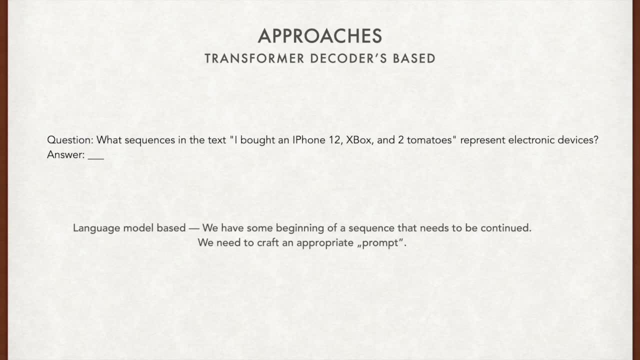 of a given text. If we provide some initial context, they will add next-probable tokens to it. writing a completion of the input sequence If we construct the input appropriately, for example, simulating the Q&A session, marking the question and finishing our context with. 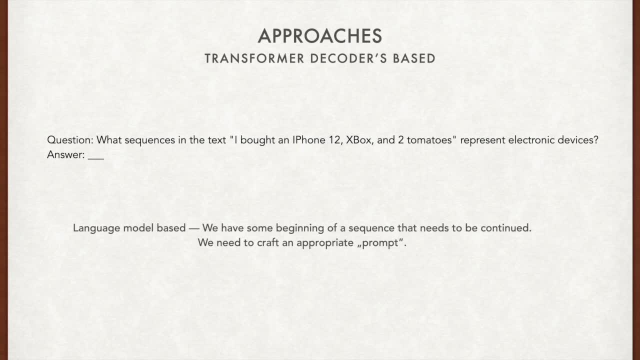 the answer word, we might encourage the model to provide an appropriate answer to that question, Considering the following example: question: what sequences in the text: I bought an iPhone 12, Xbox and two tomatoes represent electronic devices and following this with the word answer the. 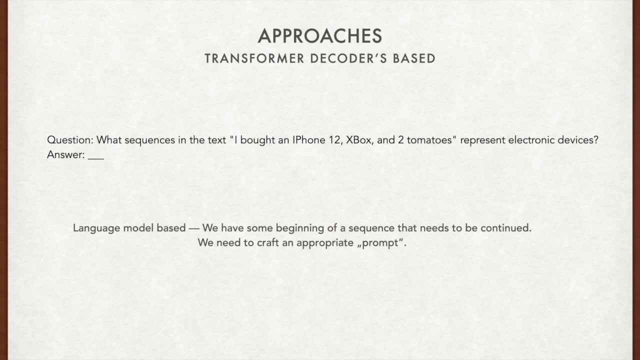 next probable words will be most probably the words representing the answer. Finishing our context with the word answer might encourage our model to provide an appropriate answer to that question. If we do this, the model will be able to generate continuations of the answer to that question, because this is the most likely continuation of the input. 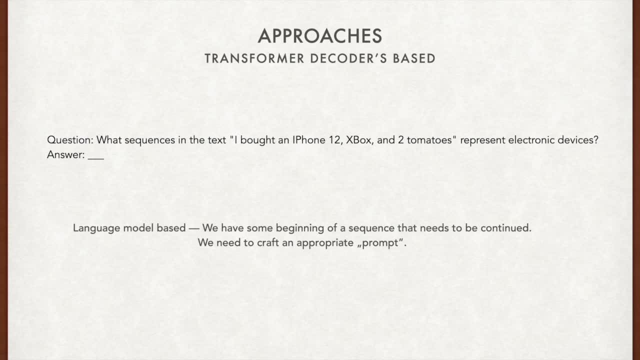 This way, we can use GPT-2,, 3 or 4 to generate answers similarly to ChatGPT or FlunT5,, but this is something that we will focus on later, When we look at the ranking provided on nlpprogresscom. 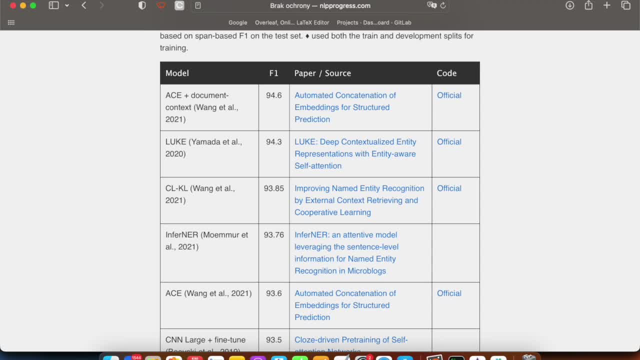 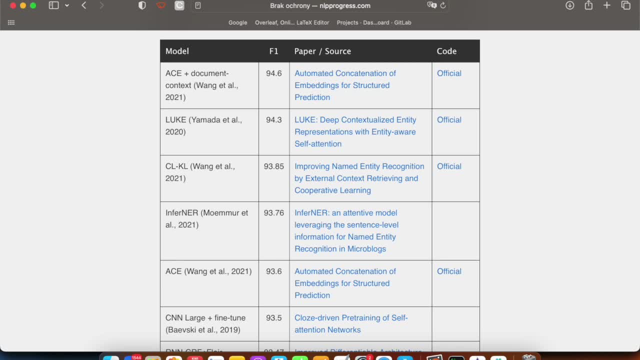 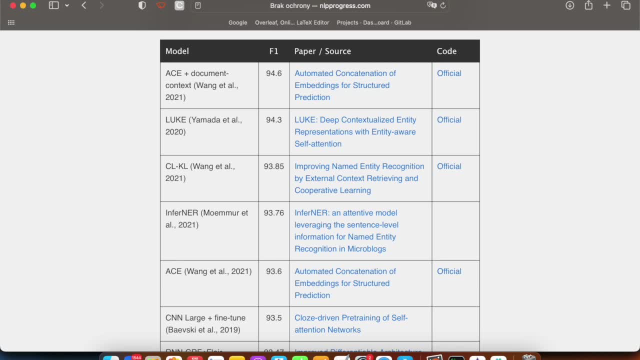 they require a lot of memory and might also be quite slow because of the number of computations involved to produce embeddings. For example, BERT large contains 340 million parameters. Alternatively, LSTM with CRF-based or FLARE-based models are also very good. 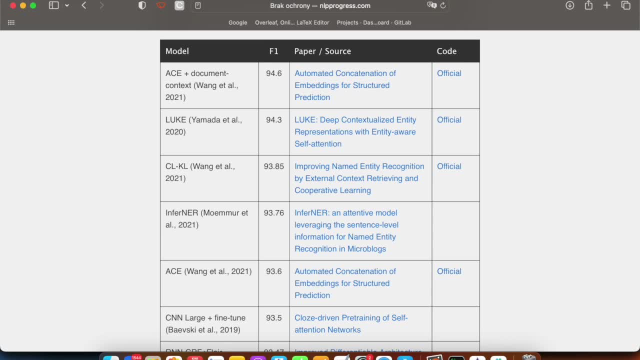 They do not provide the best possible quality, but they don't produce bad results. Moreover, they might be more lightweight and quick than look or BERT-based solution. The decision on which model to use must be based on an analysis of what code you are using, If you. 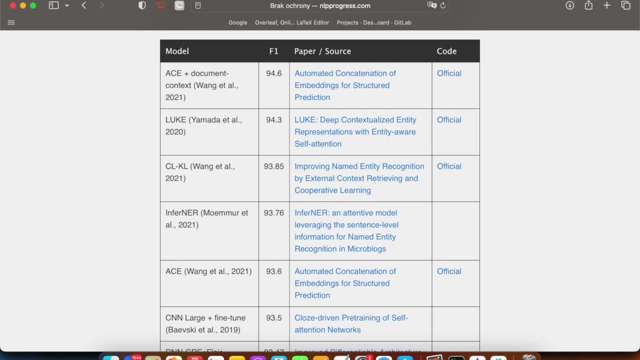 want to know more about this, you can click on the link in the description of this video. Now, as we know several approaches of solving named entity recognition task. we should discuss the evaluation metrics, because here the situation is a little bit more complex than in the case. 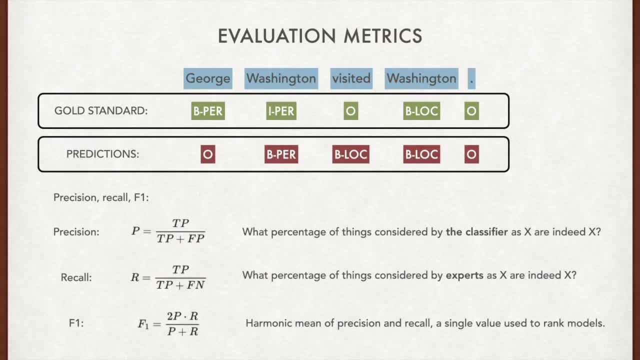 of document classification Similarly to regular classification. the most popular evaluation metrics are precision, recall and F1 score, So that we will focus here on these metrics. For each sequence in the evaluation phase, we have the expected labels encoded using a selected tagging scheme. Here we use BIO, or more precisely BIO version 2.. 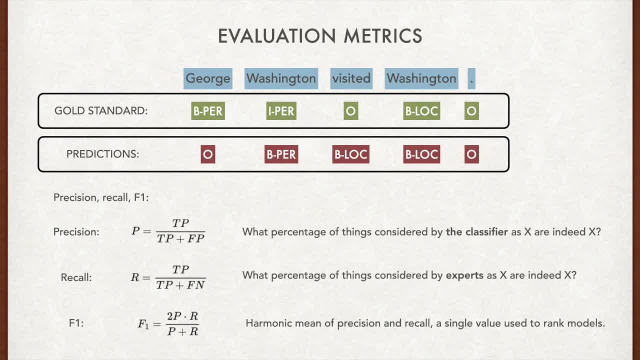 Also, the predictions made by our model are also described using BIO format. Next, we have to decide whether we would like to use BIO format or not. Next, we have to decide whether we would like to use BIO format or not. Next, we have to decide whether we would like to use BIO format or not. 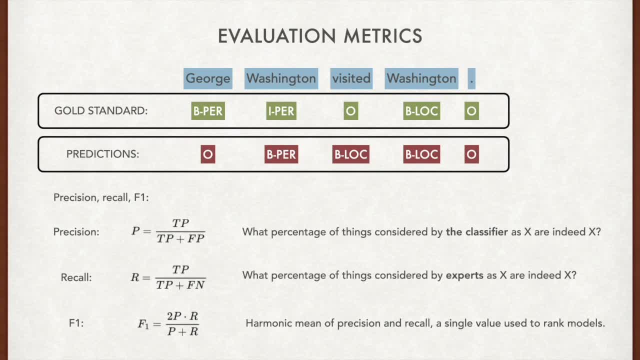 Next, we have to decide whether we would like to evaluate the model on token level, comparing all labels with prefixes included, or to form full entities first and then compare those entities. In other words, we have to decide whether we compare the tokens with the bio labels. 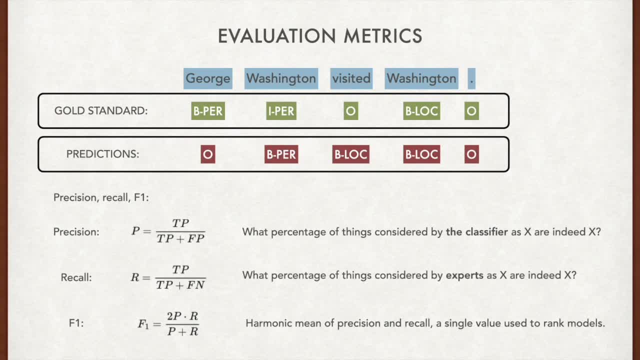 whether the first token, Georg, obtains the B person and then whether Washington obtains the label I person or whether we want to check whether the entities- the George Washington- was extracted from the text regardless single tokens and prefixes assigned. We start our analysis with the first interpretation. 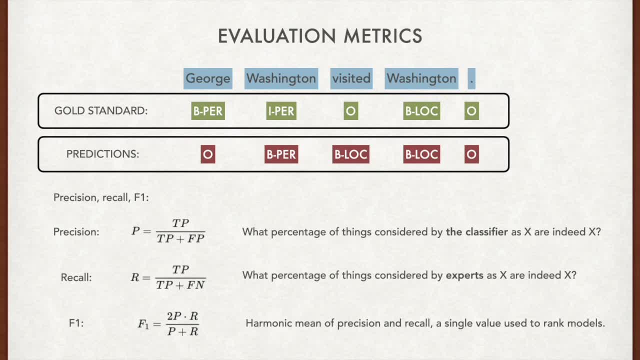 where we compare all labels with prefixes, those labels that we see here in this slide. Now let's briefly summarize how Precision, Recall and F1 score are built. These are metrics defined for each category separately. where a given category analyzed, is called a positive. 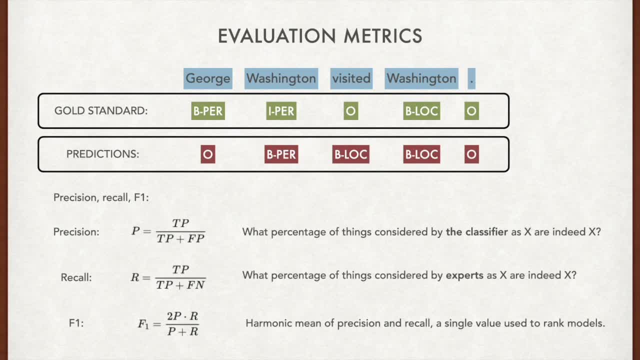 class and all other categories are called negative ones. For now, assume that our category is the label bper, which is our positive class From the perspective of the metrics described. we need to discuss three scenarios in which the bper label is mentioned. 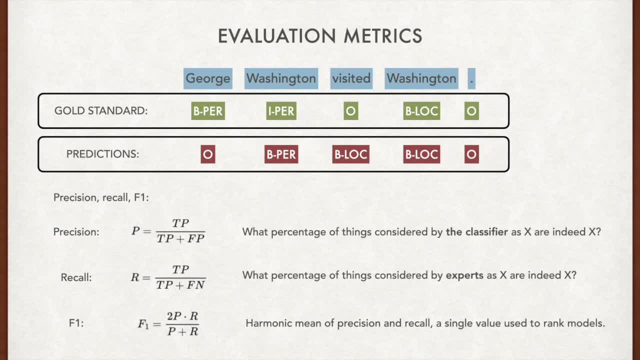 First, the true positive scenario is considered. when, at a given position, the expected label is bper and our model assigned the label bper, then we assigned the label correctly. We call that true positive because the model provided the true answer and because we calculate the. 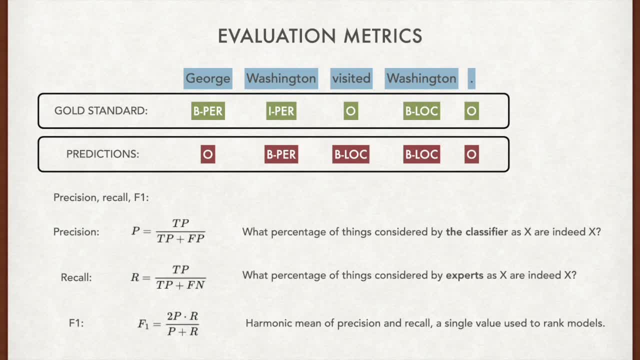 metrics for the bper label. this label is called a positive label. We would like to generate as many true positives as possible, but we don't have enough time to do that, So let's start with the true positive scenario. First, the true positive scenario is considered. 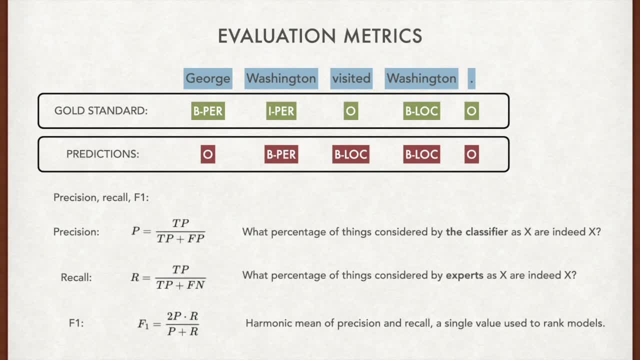 when a given token should be assigned with the bper label, which is our positive class. We will also make some mistakes here. We will make some mistakes in this scenario. There might be two kinds of mistakes. First, called false positive, occurs when a given 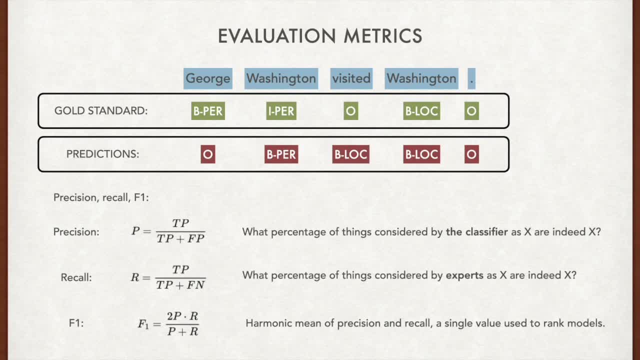 token should not be assigned with the bper label, but our model thinks it should be. It falsely assumes that the positive class should be true here, So we call that case false positive, or fp for short. Similarly we also have false negatives If a given token should be assigned with the 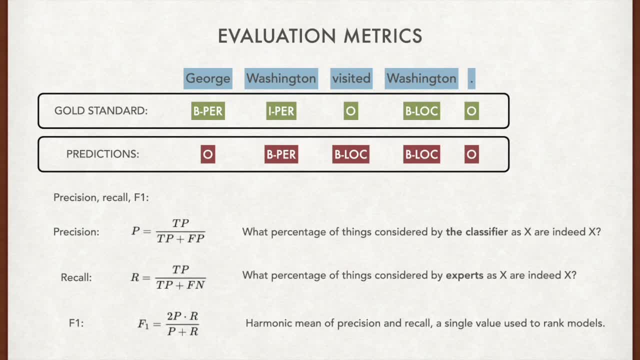 bperl label, but our model classifies it to another class. we have a situation we call false, negative or fn for short. Here we falsely assume that a given token does not represent the positive class, or in other words, we falsely assume that a given token represents. 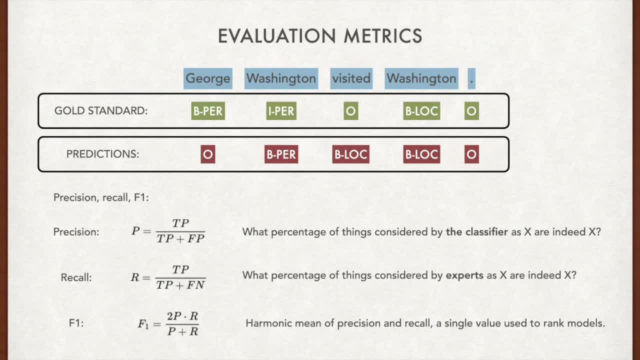 some negative class. Those distinctions can be then used to introduce two auxiliary measures: precision and recall. Precision is a single number representing the ratio between the number of true positives and the sum of true positives and false positives. This can be interpreted as from all situations in which 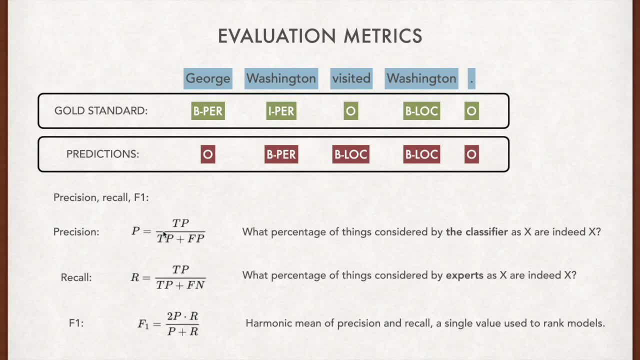 our target token is assigned with false positives, or fn for short, This can be interpreted as from all situations in which our target token is assigned with false negatives, or fn for short. This can be interpreted as from all situations in which experts assigned a given positive class. how many of them are indeed representing? 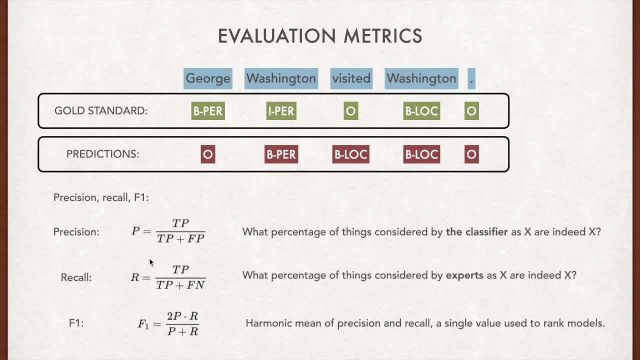 that positive class, Similarly recall, is a single number representing the ratio between the number of true positives and the sum of true positives and false negatives. This can be interpreted as from all situations in which experts assigned a given positive class. how many of them? our classifier? 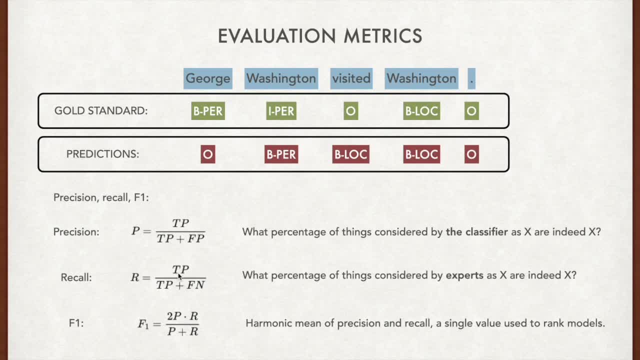 recognized correctly. Both precision and recall are numbers, the values of which fall between 0 and 1.. Frequently those are aggregated into a single number, the F1 score, which is the harmonic mean of precision and recall. As a consequence, 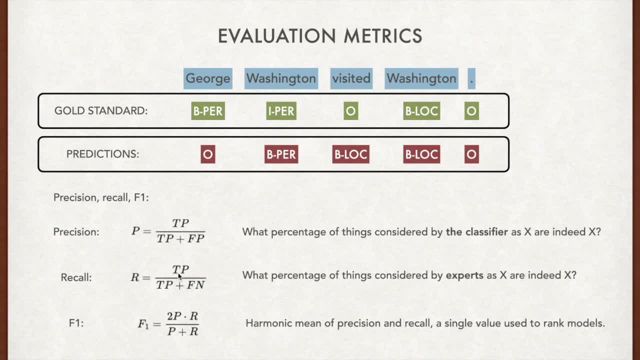 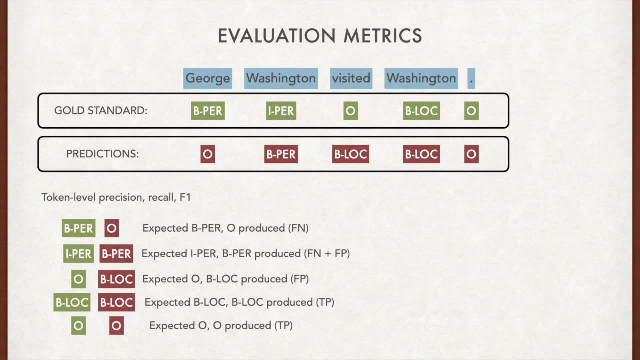 the F1 score is also a number between 0 and 1.. To check how many true positives, false negatives and false positives we have in a token-level evaluation for each category, we compare pairs of labels as presented here In the context of the. 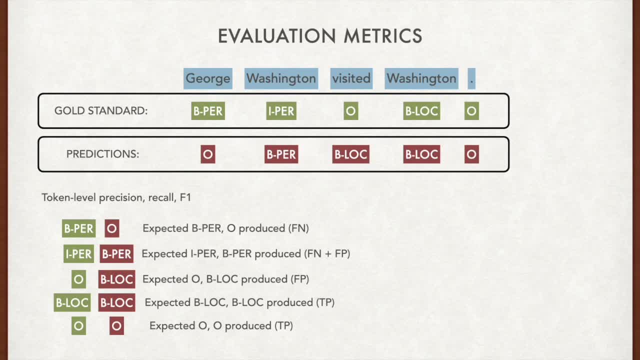 first token, George, we expected the label bPAR, but produced O. We generated a false negative, assuming bPAR to be a positive class. Comparing labels related to the second token, we generate bPAR instead of IPAR and this way we produce both a false positive and a false negative From the perspective. 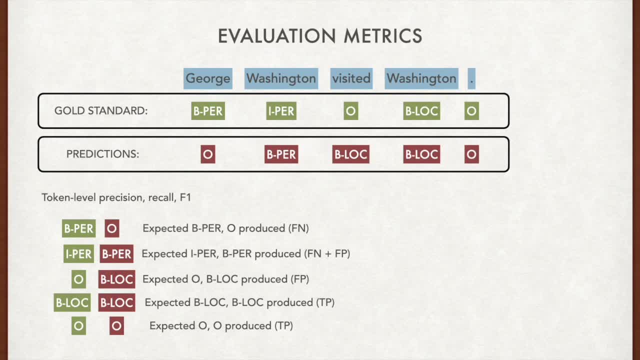 of the IPAR label as a positive class. we generated false negative. We expected IPAR but generated something different From the perspective of the bPAR label assigned by our tagger. we generated a false positive. We falsely assumed that the positive class 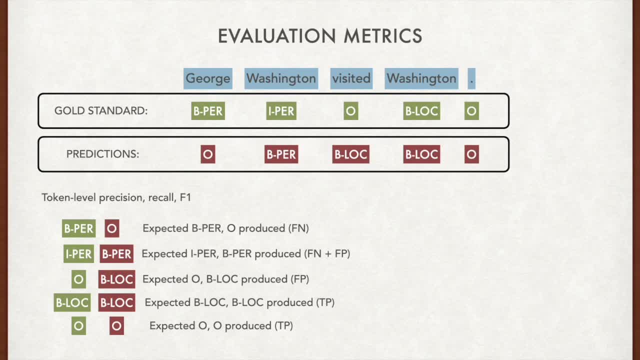 here is bPAR. During the third token, we generated a false positive because we did not expect bLog to be here, And in the context of the fourth token, we generated a true positive because the positive label- bLog- was detected correctly. Please note that we don't calculate metrics. 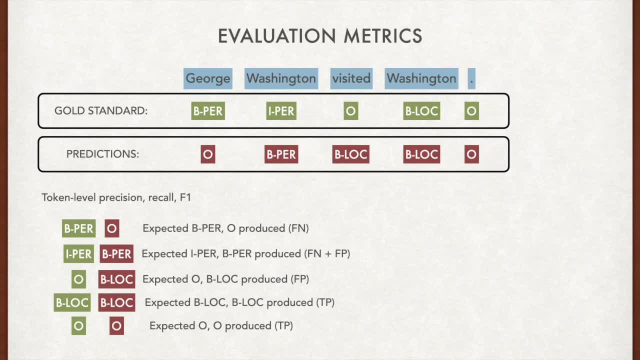 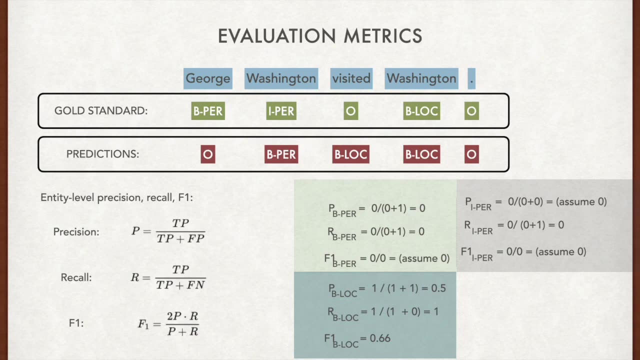 for the O label because it does not represent any of our entities And those observations can be used to calculate metrics. The precision of bPAR is equal to 0. We never produced a True Positive here, but generated one false positive related to the second token. Similarly, the recall is also 0, we 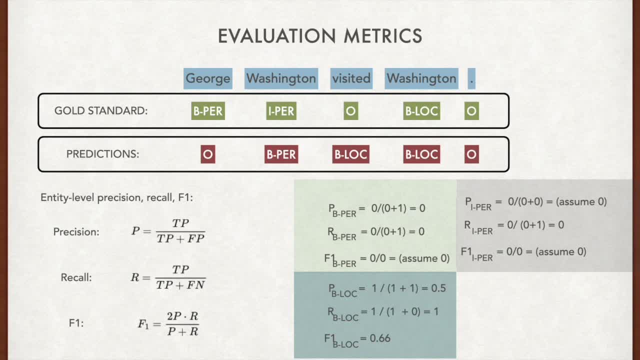 have no true positives but one false negative related to the first token in our sequence, F1. FTISDA has negative unlike f1measure, which means it is positive. The F1 measure is 0 divided by 0. Let's assume that it is zero. 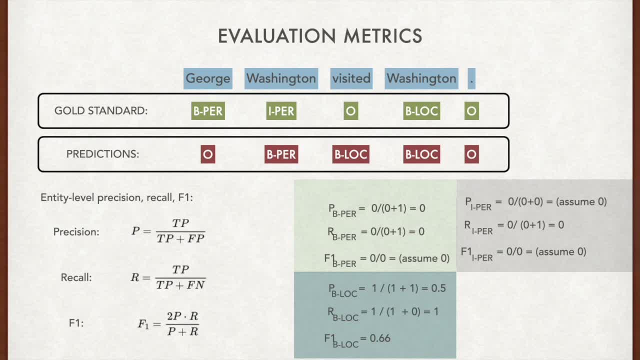 We'll assume that it is a face value as a factor And since areroom values are 0,, we are left with exactly 20.. At the same time, the microwave- there is claims, the precise is 0.. Considering the IPer as the positive class, the precision is also 0,. our attacker, 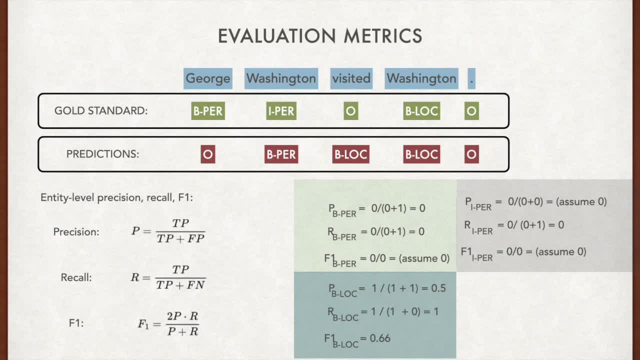 never produced such a label, so that we didn't produce any true positives or false positives, The recall is equal to 0, because we produced a false negative in the context of the second token and no true positives, So the F1 score is also 0.. Finally, if we consider the BLOCK, 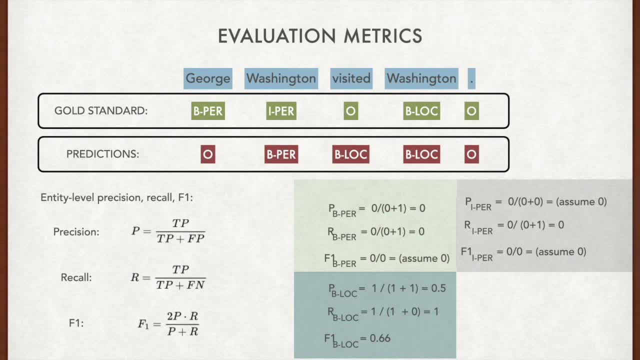 label as the positive class. we can have one true positive case related to the word WASHINGTON and one false positive related to the word VISITED. Thus, the precision is equal to 0.5 and the recall is equal to 1.0.. The harmonic mean between these is 0.66.. 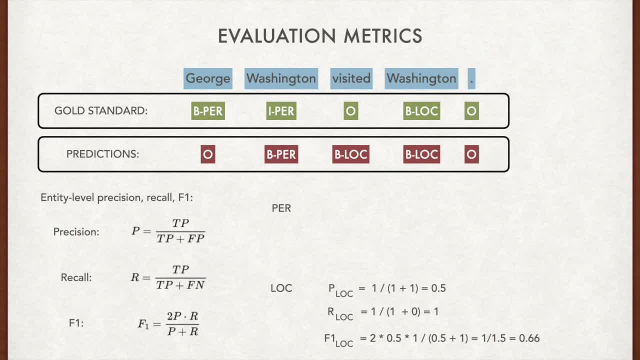 However, instead of calculating the matrix for each token in our sequence separately, we could identify the 원 in both cases and we can generate a final value of 0.66 of four, identify whole entities, possibly multi-token entities, and then compare full entities. 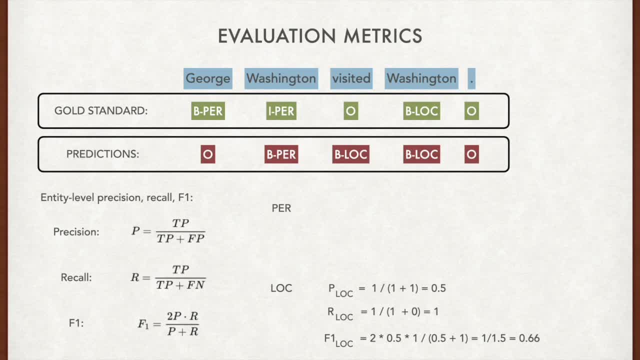 those expected with those generated, without splitting them into separate tokens and comparing bio-prefixes. In the slide shown here, the locations expected and produced are single tokens, so that the calculations of related metrics will be exactly the same. The B-Log label represents, in this example, the whole location, so the metrics are the. 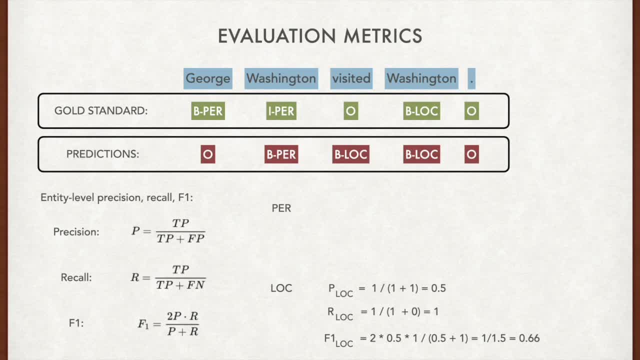 same. However, from the perspective of George Washington, the situation is more complex. The whole George Washington represents a single person. This way, we might have three cases to consider. The produced entity In the first case is strictly the same as the expected one, covering exactly the same. 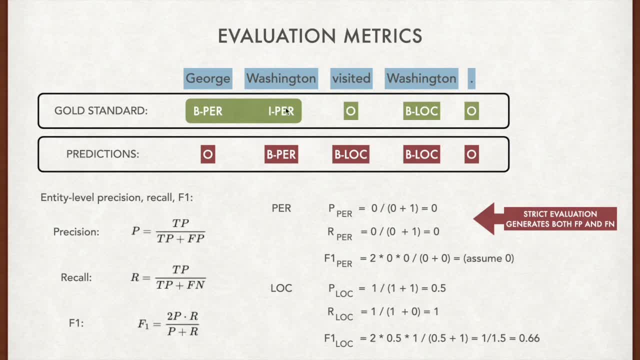 sequence of tokens here: George and Washington. However, the produced entity might only overlap with the expected entity, like in this case. We expected George Washington to be extracted, however, our model extracted only the word Washington. Finally, we can produce an entity that is disjoint with the expected entity. 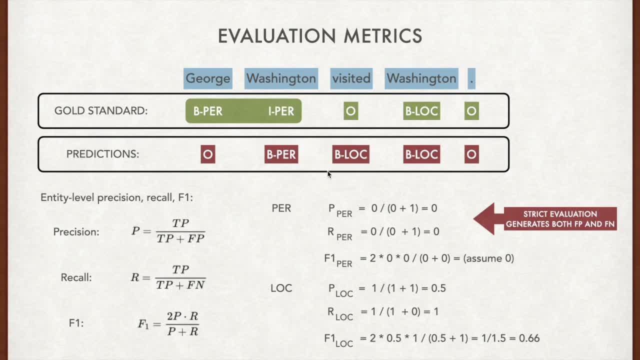 The first and third scenarios are quite straightforward. however, the second one requires making some decisions. We can assume that we apply a strict evaluation. A true positive is generated only when the entity consists of exactly the same sequence of tokens as expected and we don't allow to introduce even minor errors. 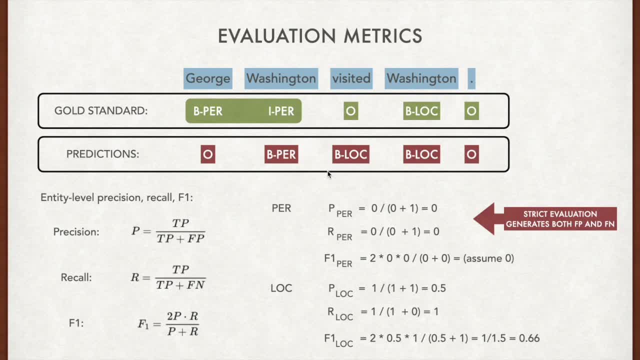 Then we expect that the whole George Washington is tagged as a single entity of the person type. Under that assumption, we have no true positives related to persons. because we didn't extract the whole George Washington, However, we have both a false positive and false negative. 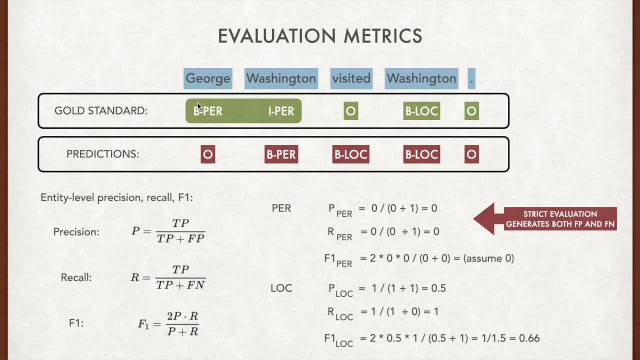 False negative because the expected George Washington was not extracted and false positive because instead we generated Washington entity that was not expected as a separate entity. As a result, the precision, recall and F1 scores are equal to zero. However, we could also weaken those requirements. 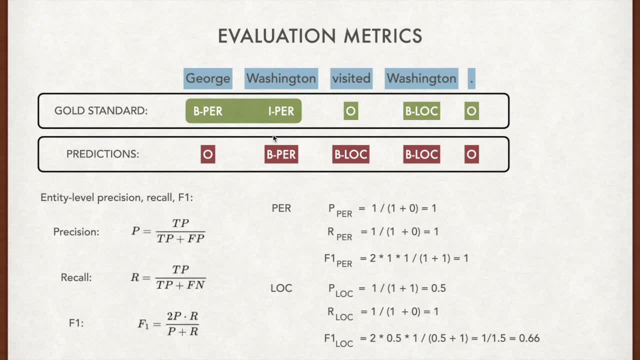 We could say, for example, that we consider a true positive a situation in which the generated output overlaps with the expected one, assuming that the appropriate class is detected. Here we can decide whether it is enough to have some overlap or if at least 50% of tokens. 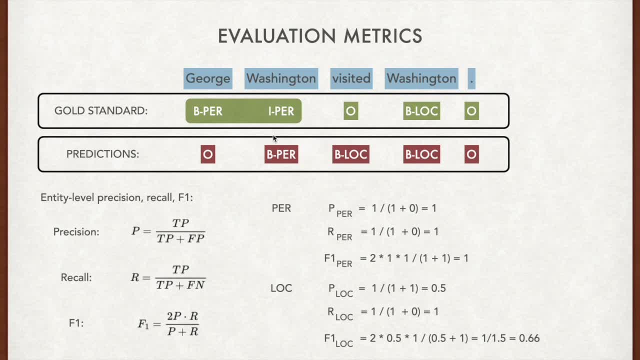 should overlap to consider it as a true positive. Under the weakened restriction, we could treat generating a person called a true positive as a true positive. For example, we could consider a person called Washington as a true positive because that token overlaps with the expected George Washington entity and the generated entity covers 50%. 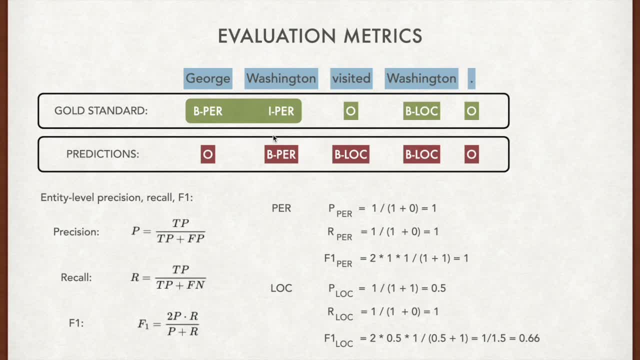 of the expected string. In that scenario, our metrics increase so that we have only true positives. One small change changed the scores completely. however, because of this variety of interpretations we have, We have to document our decisions, specifying what things we considered as true positives. 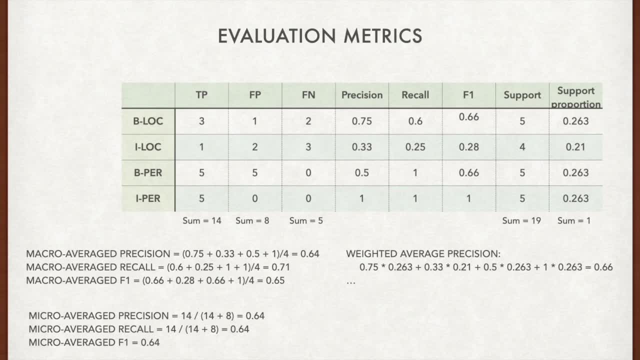 Having precision recall and F1 scores calculated for each entity type or each label with bio-, below- or bio-is-prefixes can help understand the weak points of our tagger. However, when comparing two algorithms, we would prefer to have a single aggregated precision. 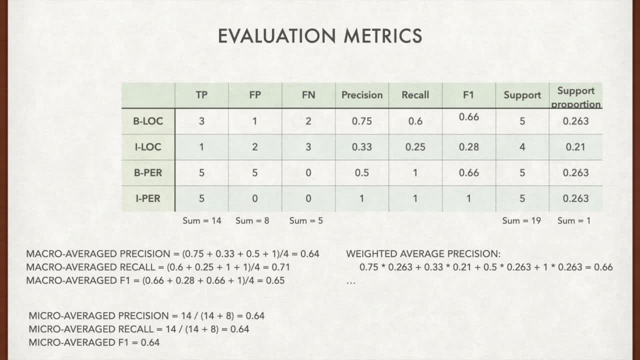 recall and F1 score to be reported Here. some aggregations can be proposed to aggregate scores related to all categories into a common number. The first one is called macro-averaged score. It can be applied to precision, recall and F1 score. 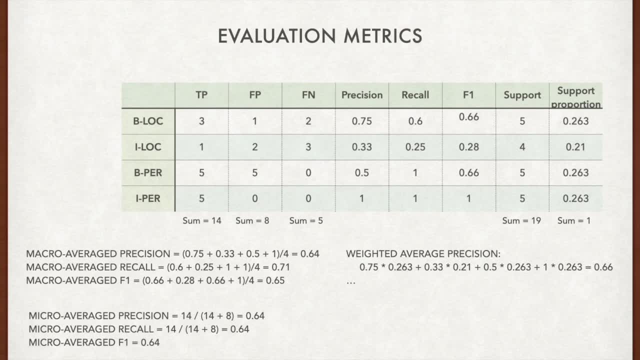 To calculate macro-averaged score. we simply calculate the average of the metrics we focus on. The macro-averaged precision is then the average of the precision related to each label. The second one is called micro-averaged score. Here, instead of calculating averages, we calculate the total number of true positives, the total. 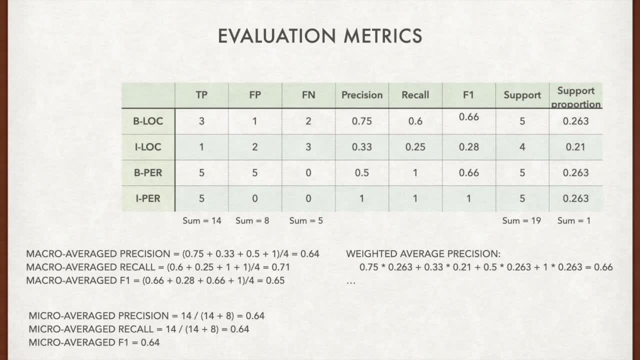 number of false positives and the total number of false negatives generated. in our system. We use such global information to calculate the average of the metrics. The average of the metrics is the number of true positives, the total number of false negatives, the total number of false negatives and the total number of false negatives generated. 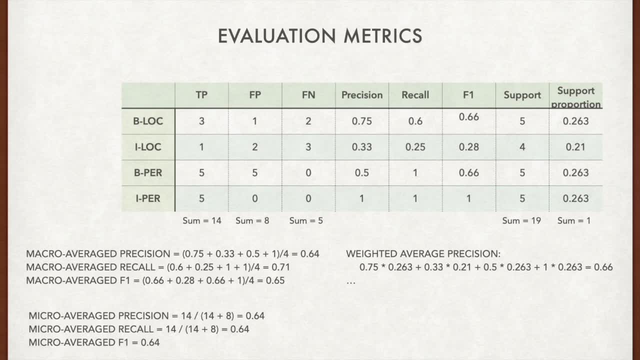 in our system. Finally, we can have weighted precision, weighted recall and weighted F1 score. Each category has a given number of examples marked by the expert in the test set. For example, the total number of tokens marked as BLOCK by the expert is equal to the sum. 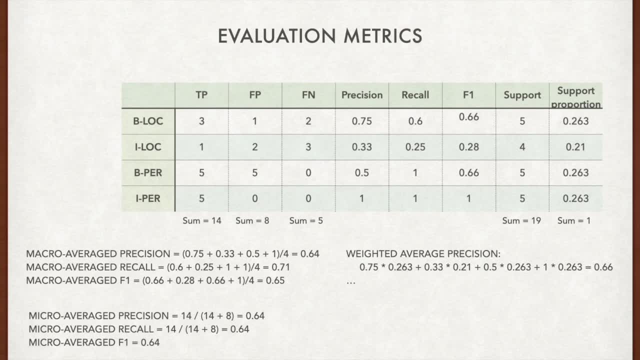 of true positives and false negatives. The number is called support. We can use supports to calculate the weighted average of the metrics. Here we calculate the weighted precision After we calculate the proportions of our supports by dividing each support by the sum of all supports. we multiply appropriate precision related to a given class by the support proportion. 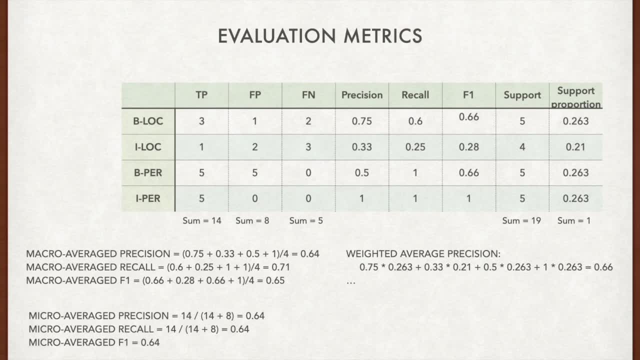 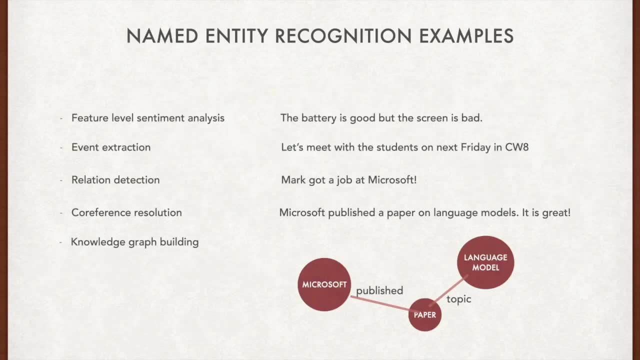 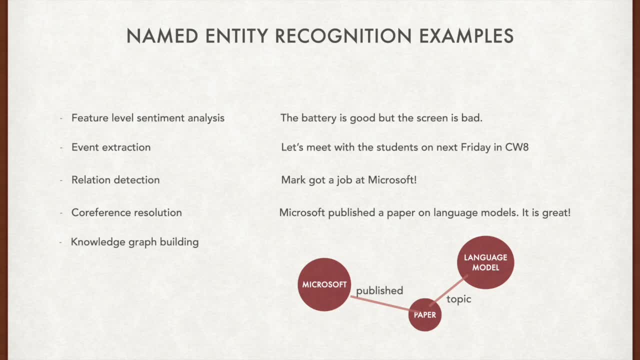 The first one is the Future Level Sentiment Analysis. This task focuses on automatic analysis of the emotions related to given features in textual documents. Imagine we run a company producing smartphones. We can try to produce an application that will find features related to our smartphones. 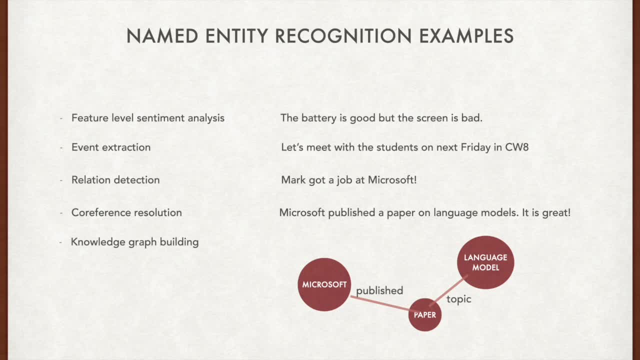 using named entity recognition models and we can call those features, aspects. These aspects might be the following: might be, for instance, the battery, the screen or operating system, And our application could try to relate emotions to those features, those aspects. In a review provided in the 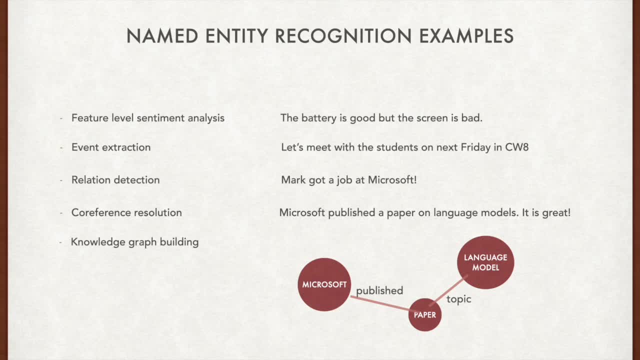 internet, we could detect automatically how people react to our battery, whether they react to our battery positively, but maybe they react negatively to our screen. Another possible application of an entity recognition model is the event extraction task. If we manage to detect dates, mentions about persons and locations we could assume. 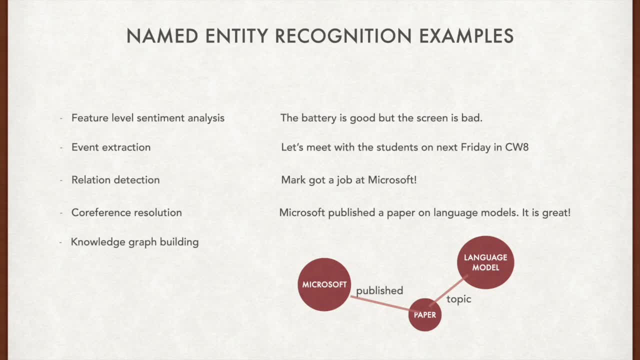 that if those information are presented close to each other, they might represent events, as each event has some participants, some date and some place. We could even try to detect relations between interesting fragments of texts Here. the entities extracted using the named entity recognition model might be classified together. 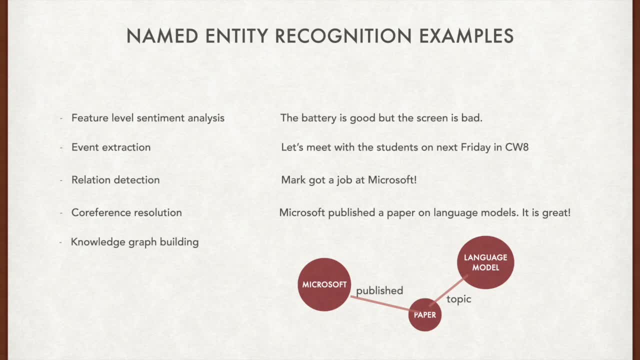 to detect what relations are there between those entities. As we can see in this slide, if we extract the entities marked and Microsoft, we could relate those entities with works at relation. Named entity recognition would be also useful in the context of coreference resolution. 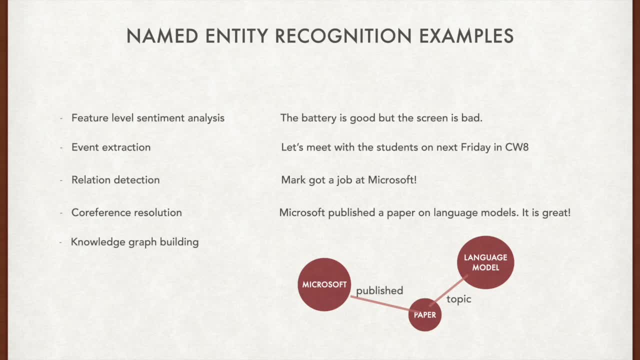 In that task. our goal is to detect which pieces of text refer to the same entities. Here we should be able to detect that the word it refers to the entity paper. Finally, the ability to detect entities might be used to produce knowledge graphs. These are graphs with entities in the nodes and relations between. 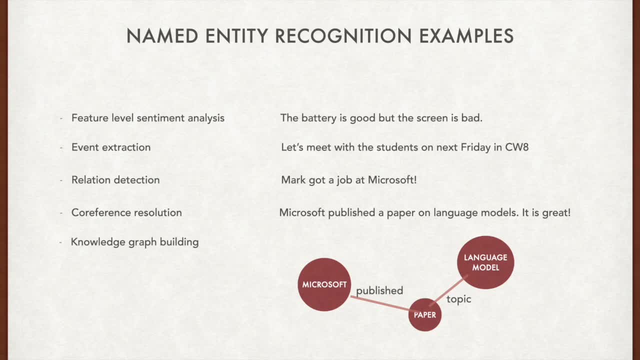 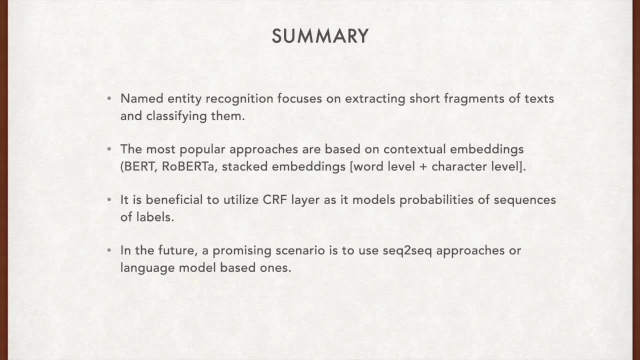 them. It can be useful in the context, for instance, of question answering systems. And this concludes our lecture. Today we learned what is named entity recognition task: why do we need it, what are the popular approaches and how we can measure the quality of the model. 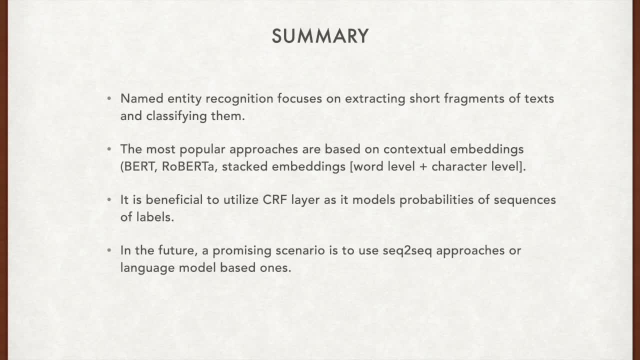 As well as how we can encode the labels. We see that named entity recognition focuses on extracting short fragments of texts and classifying them. The most popular approaches are based on contextual embeddings, Baird-based, Roberta-based stacked embeddings, utilizing word-level and character-level embeddings. 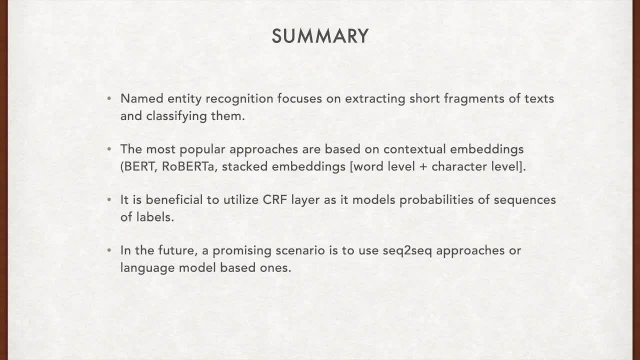 Also, we see that it is beneficial to utilize CRM. It is interesting to note that the transaction queries in CRM are not just about a set of words. On the other hand, it is useful to compute the most common method of information transfer in CRM. 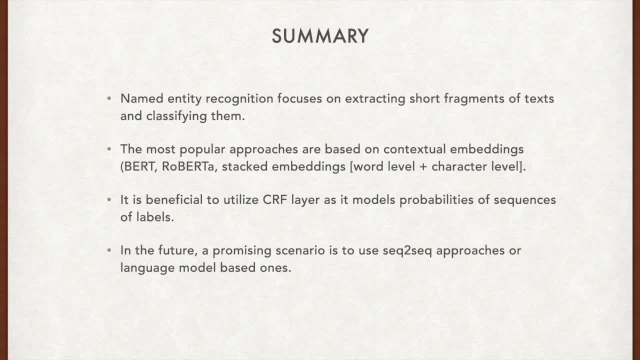 First let's look at the model of the CRF layer As it models probabilities of sequencers of labels. So we can not only focus on the representations of tokens, but we can also focus on the sequences of labels. In the future, a promising scenario is to use seek-to-seek approaches based on transformer.